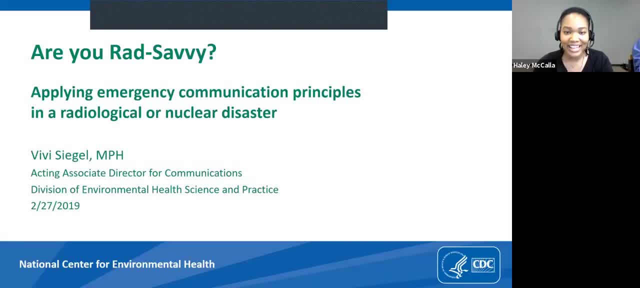 Good afternoon. My name is Haley McCalla and I'm an ORISE fellow appointed to CDC's Center for Preparedness and Response Division of Emergency Operations. Thank you so much for joining us for today's epic webinar titled Communication for a Nuclear or Radiological Event. 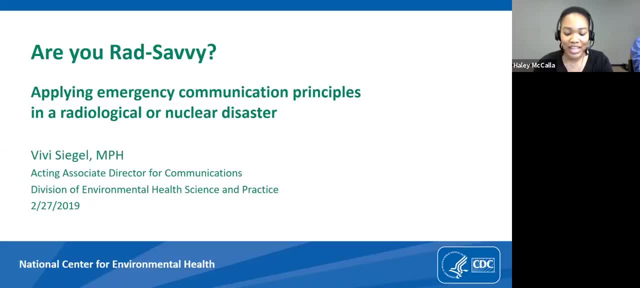 Today we will hear from Vivi Siegel. If you do not wish for your participation to be recorded, please exit at this time. You can earn continuing education by completing this webinar. Instructions on how to earn continuing education can be found on our website. emergencycdcgov- slash epic. 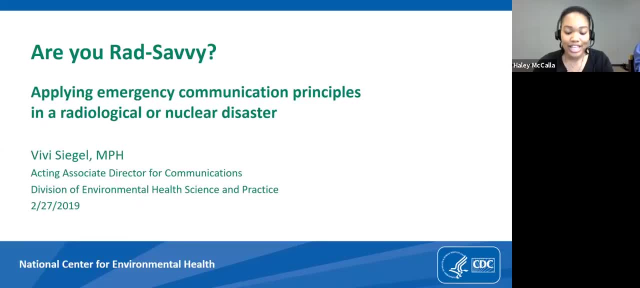 The course access code is EPIC0227, with all letters capitalized. To repeat, the course access code to receive continuing education is EPIC0227.. Thank you. Today's webinar is interactive. To make a comment, click the chat button on your screen and then enter your thoughts. 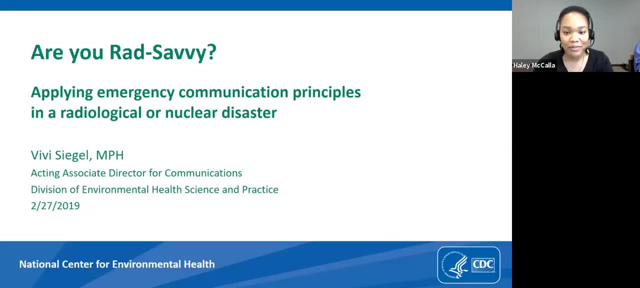 To ask a question, please use the Q&A button. The Q&A session will begin after our presenter has finished. Closed captioning is available for this webinar. There should be a button on your screen for you to enable this feature. We are very fortunate today to have Vivi Siegel as our speaker. 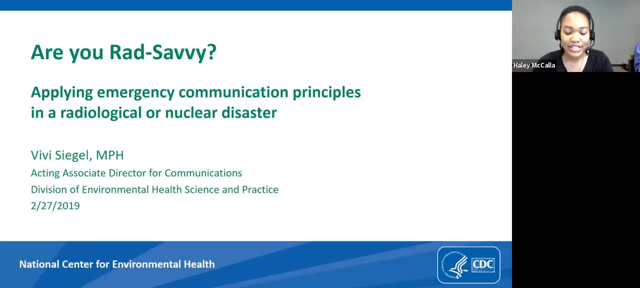 Vivi Siegel is the Acting Associate Director for Communications for CDC's Division of Environmental Health Science and Practice. Vivi has a background in public health and journalism and a professional focus on emergency risk communication and environmental health. She has been a health communications specialist at CDC since 2005.. 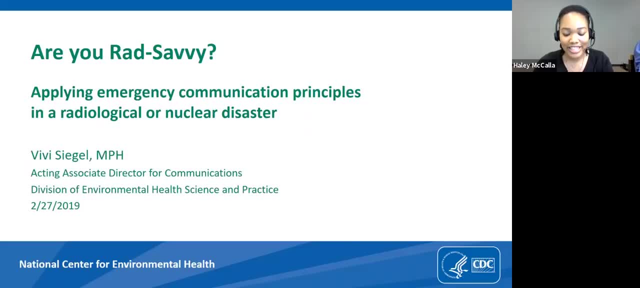 She helps lead communication responses for natural, chemical and radiological disasters, including the 2001 earthquake. She also led the 2011 Fukushima response and 2017 National Gotham Shield exercise. Thank you so much for joining us today, Vivi. 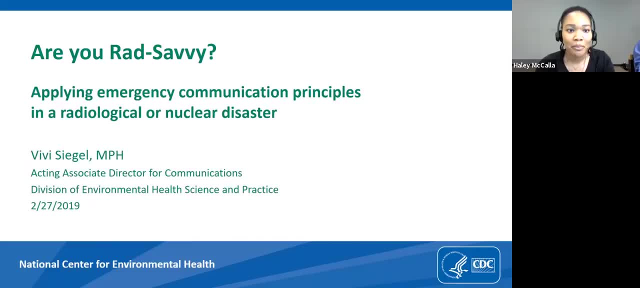 Please begin. Good afternoon to everybody joining us from the East Coast, Good morning if you're calling in from another part of the country, or good noon. Thank you, Hailey, for the introduction. We really appreciate everyone being here today and taking a little bit of time to chat with you. 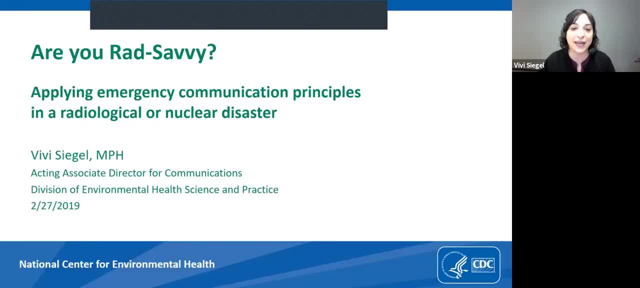 And taking a little bit of time to talk with us about this topic And, like Hailey said, I'll be answering questions at the end- And today I really want to talk with you about how we might apply emergency communications principles that we are used to applying for natural disasters or other types of common emergencies. 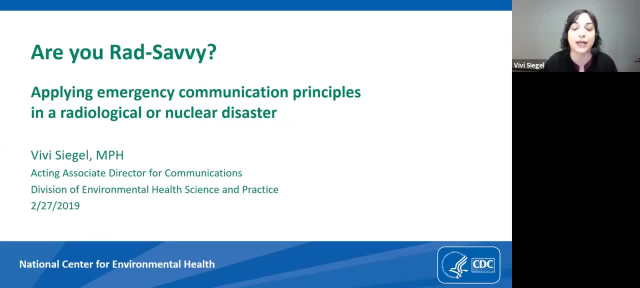 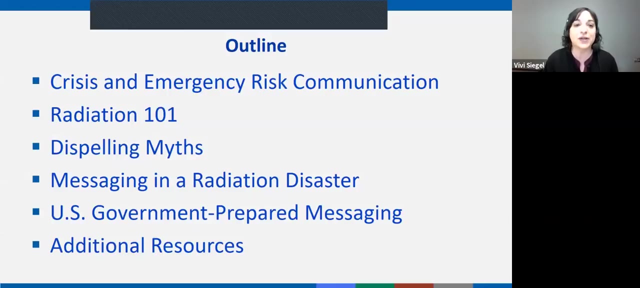 to something that is hopefully much less common and that would be a potential radiological or nuclear disaster. So, Hailey, we'll be moving the slides today, so, if you don't mind, we'll start now, Thank you. So first we'll talk a little bit about CDC's crisis and emergency risk communication principles. 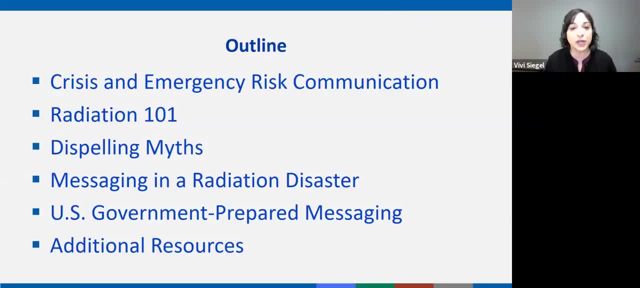 And if you've been on some of these EPIC webinars before, you probably are familiar with this, Or if you work within communication or emergency communication in your jurisdiction, you may be familiar with this, And these are the principles that CDC uses in our own emergency communications. 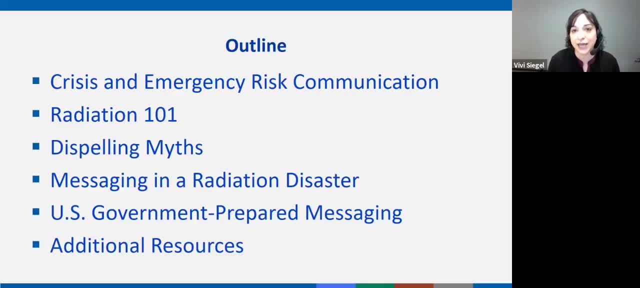 And really find that they help us in communicating difficult and uncertain information to people. We'll talk a very little bit about radiation basics. I am not a health physicist, I am not a radiation expert, So my approach to radiation 101 are: what are the parts about radiation that communicators really need to know? 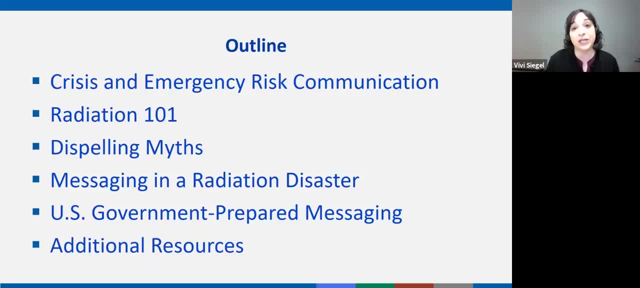 and what are the things that we need to know? we don't know before we start talking about radiation. We'll talk a little bit about common myths about radiation, Our CDC message, research about messaging in a radiation disaster, And then I'll talk about the resources that the federal government has for state and local jurisdictions. 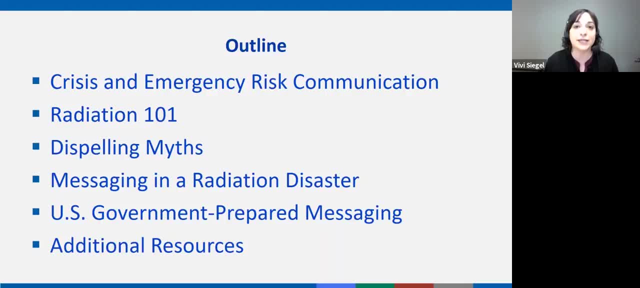 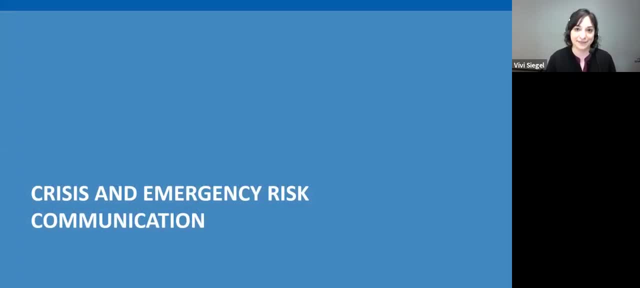 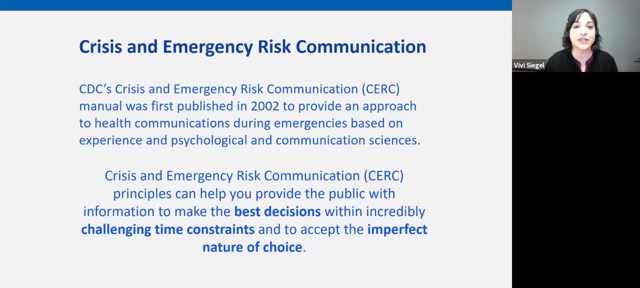 in the event of a nuclear event, and additional CDC resources that we have available. So what is crisis and emergency risk communication? This is something that CDC first developed- Dr Barbara Reynolds, in 2002, to provide an approach to health communication during emergencies. 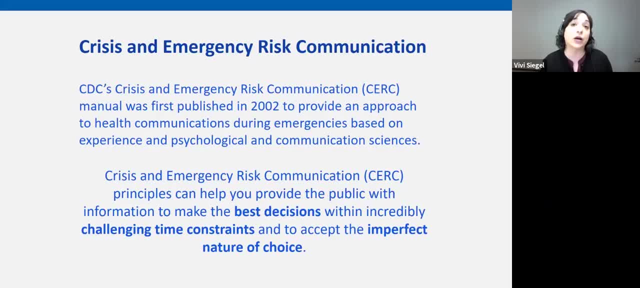 thinking about how people's psychology changes an emergency situation. So it's always difficult to talk about health topics with people, And when they are worried about their physical safety and they're worried about their family or their friends or their homes, it's even more difficult. 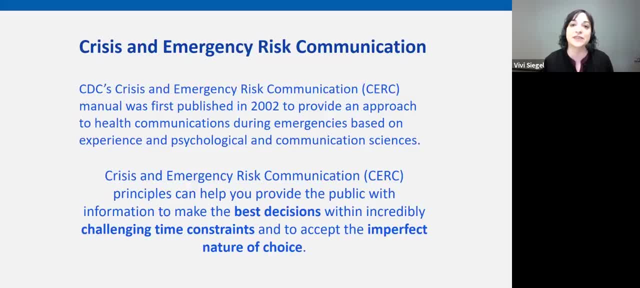 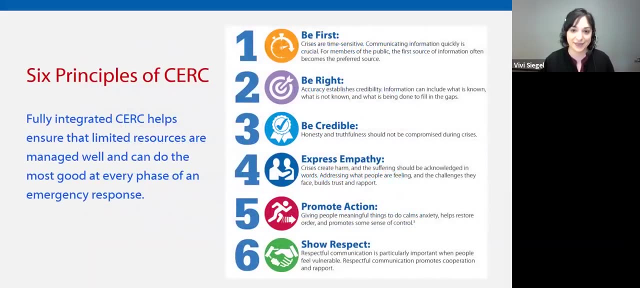 So crisis and emergency risk communication principles give us some tools to help talk with people in difficult situations and help them make the best decisions for their own health. And so here are the six principles of CERC: Go ahead, Haley. So the first one is: be right, be first. 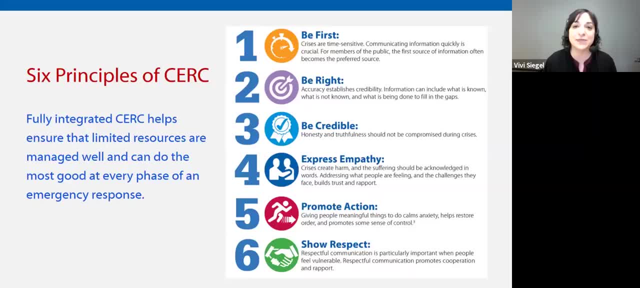 The first one is be first: Crises are time sensitive. We know that in a crisis situation, people are looking for information as fast as they can get it. These days, that's probably on Twitter- And we know that the person or organization who comes out with the first information 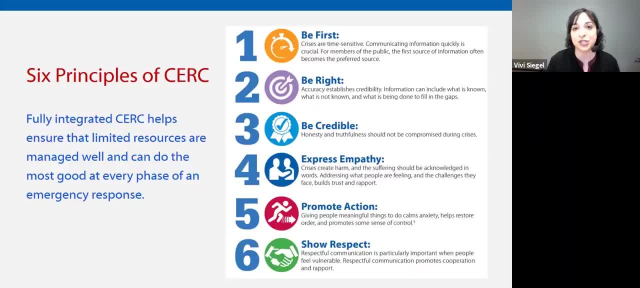 is going to be a source that people come back to. They tend to trust the first information they hear and compare everything else afterward to it. So our approach at CDC is: we know we're not going to have all of the information that people want right at the beginning. 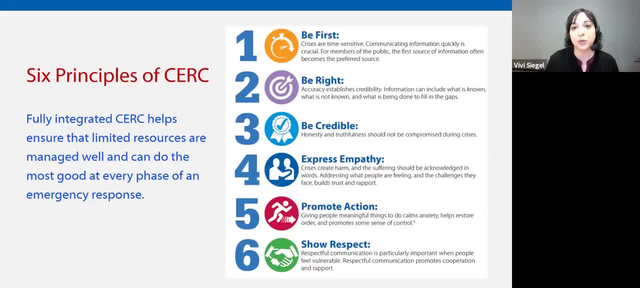 We know there are going to be questions. There are going to be questions that people have, But we think it's appropriate to say we know something happened, We're looking into it, We're finding out more And we're going to keep you updated as things progress. 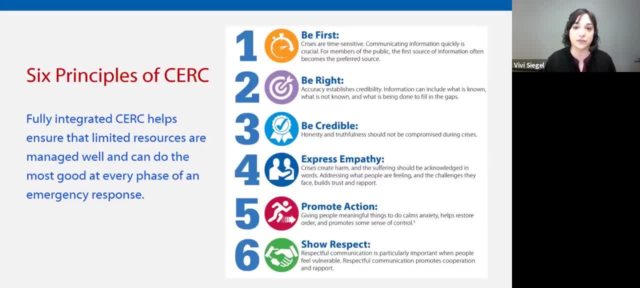 We're establishing ourselves as a go-to source of information. Second, be right. Accuracy is so important because once you lose it, you're really losing the trust of your audience. So- and that doesn't mean to say things, Say things, It means to wait and say nothing until you can verify things 100 times. 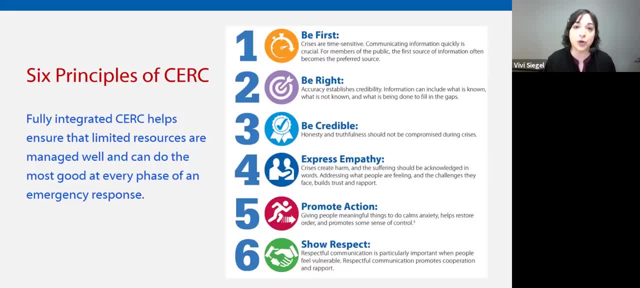 It means to say what you know, explain what you don't know and explain the process that you're using to find out holes in information. Be credible. Honesty and truthfulness should never be compromised. Express empathy And, as Dr Reynolds used to say, this is more than just having empathy, but showing your empathy through your words and through your actions. 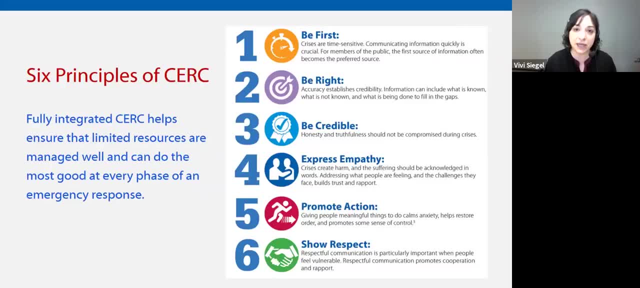 Promoting action, Giving people things to do that are meaningful And that can help them address both their safety and the mental distress that they're having. So at CDC we try, in every message that we give through our social media channels, through our media channels, to give people actionable things that they can do to help protect their health. 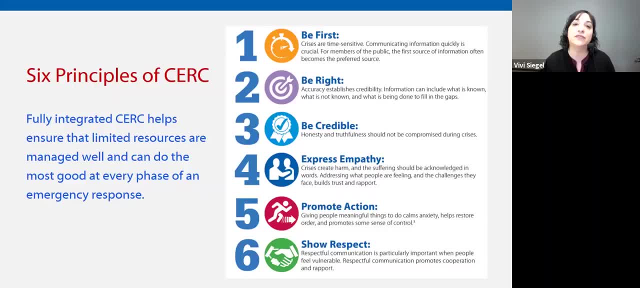 And this situation is like any other, And if you have any questions, please feel free to reach out. Thank you, Radiation emergencies are survivable and there are things that people can do to protect their health if they know what to do. Finally, we show respect. 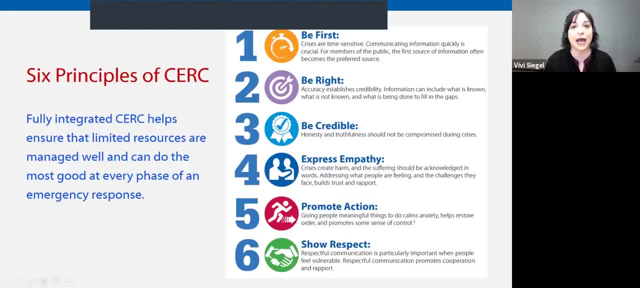 And we do that not only with our words, but with our actions and how we engage people, when we talk to them and using their languages, respecting their customs and finding people where they are And respecting their feelings and what they're going through. 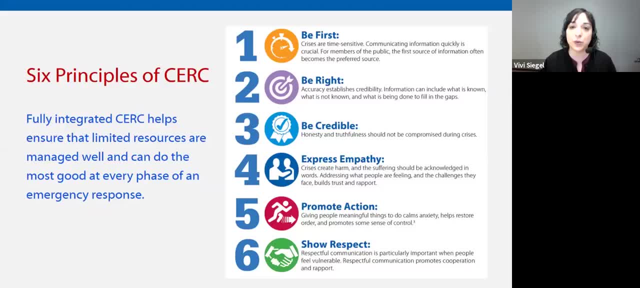 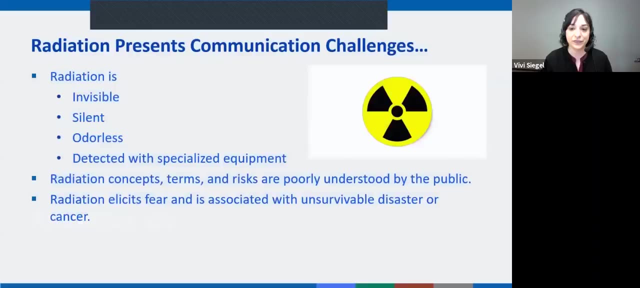 And these are tools that we use in the event or in the recovery phase for any type of emergency response. Thank you. Next slide, please, Haley. So a little bit about radiation. Why is it so difficult to talk about? And the same can be said for a lot of times when we're talking about environmental contaminants. 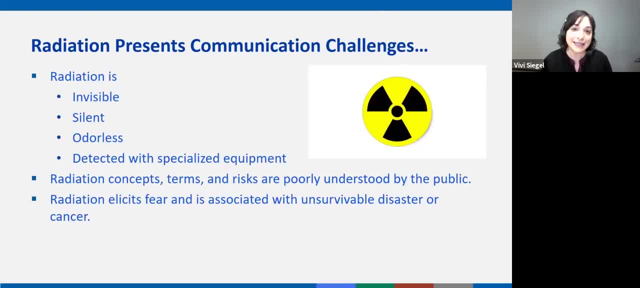 They're often invisible. They are silent. Radiation is odorless And you have to have specialized equipment to detect it. You can't just tell if it's around. That is scary to people. Radiation concepts, terms and risks are poorly understood. 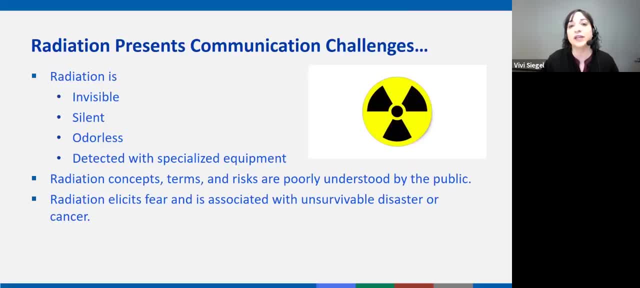 And they elicit fear. Often the education that people have had about radiation comes from comic book movies or it comes from historical events And they really don't understand. They don't understand what it means in today's circumstances. Go ahead Next slide. 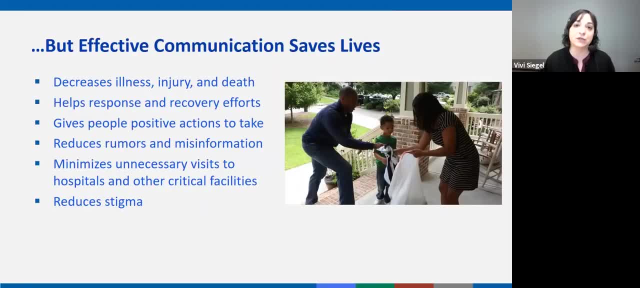 But we know that if we are able to get information to people in a timely manner, we can save lives. We can protect health. Giving people positive actions to take helps protect them and their families. It helps reduce rumors and misinformation. It helps minimize the unnecessary trauma. 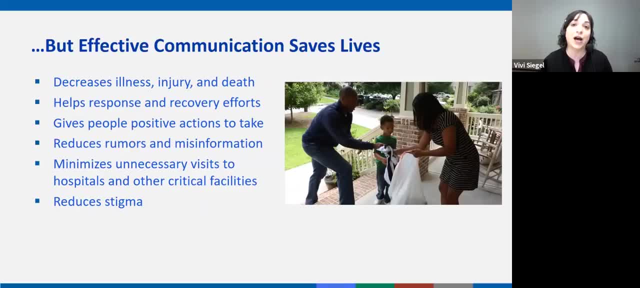 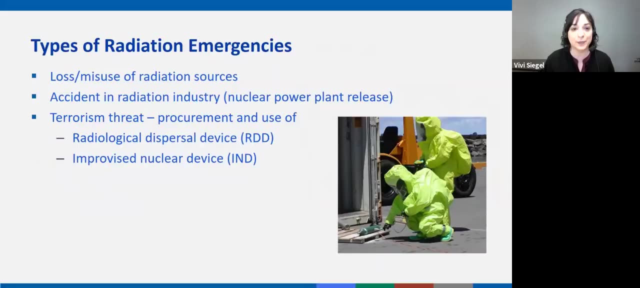 It helps reduce traffic to hospitals and clinics. People won't go if they know they don't need to, And using information correctly can reduce stigma that can follow after a disaster such as a radiation disaster. Next slide, please, Haley. So when I say radiation emergency, what do I mean? 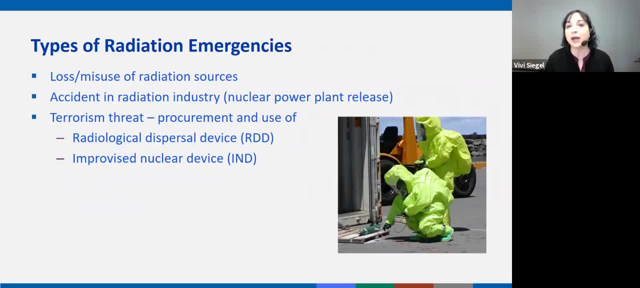 There could be a few different kinds of radiation events that we might find ourselves talking about from a public health perspective. We've heard of a loss or misuse of a radiation source, Something that might be in the transportation chain, Something on a truck, Accidents in the radiation industry, such as a nuclear power plant, like we saw in Fukushima. that happened because of a natural disaster. 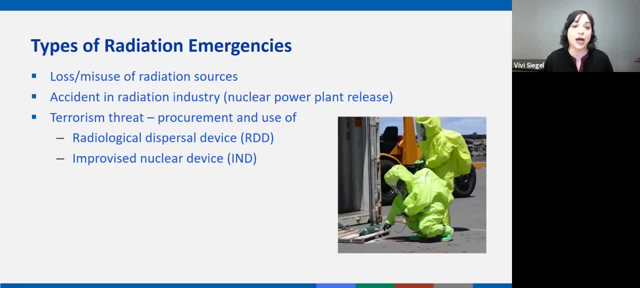 Or it could be an intentional use of radiation through a radiological dispersal device, which is something that could be, you know, something that could be used to spread small amounts of radiation, Or an improvised nuclear device, which would include a nuclear explosion which could spread nuclear energy. 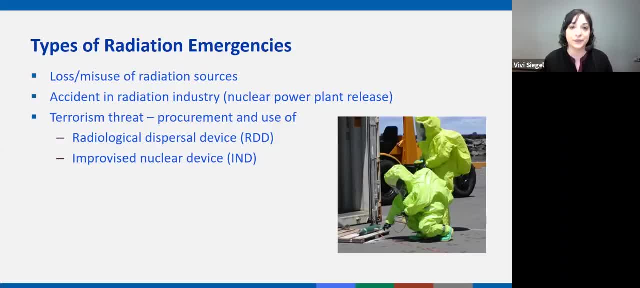 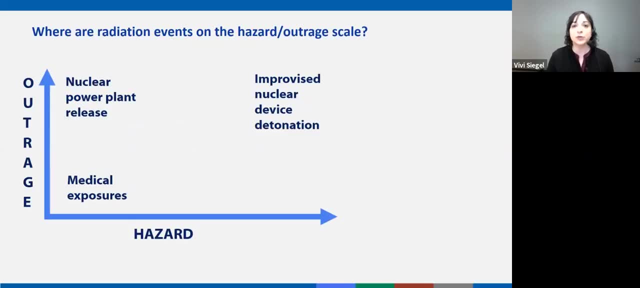 We're going to talk a little bit more about that going forward. Next slide please. And if you're familiar with some risk communication principles, you may have heard about this hazard outrage scale. that's really explained well by now. That's really explained well by Peter Sandman. 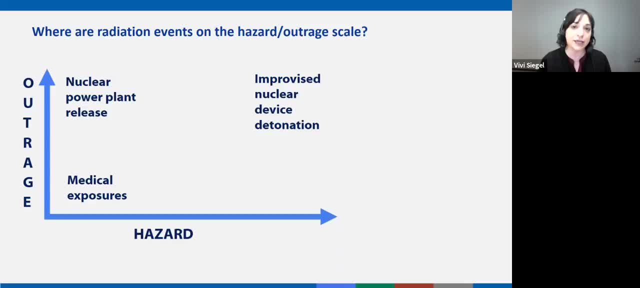 And what this means is that certain events can cause a lot more angst and turmoil for people, And it's because they have less control over what's happening. So, for example, some things match in hazard and outrage And you'll see in the bottom left corner medical exposures to radiation. 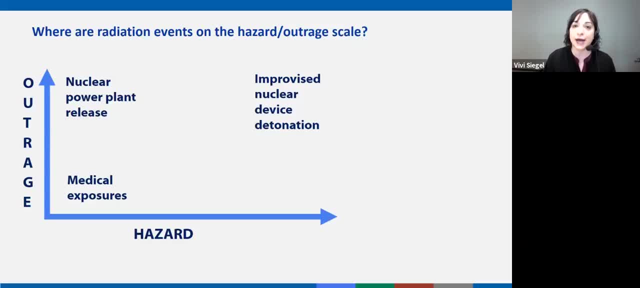 They're generally pretty low risk to people. You know, obviously the more you have, the more radiation you're exposed to. But most people aren't too afraid to go and get an x-ray And also their outrage factor for an x-ray is not very high. 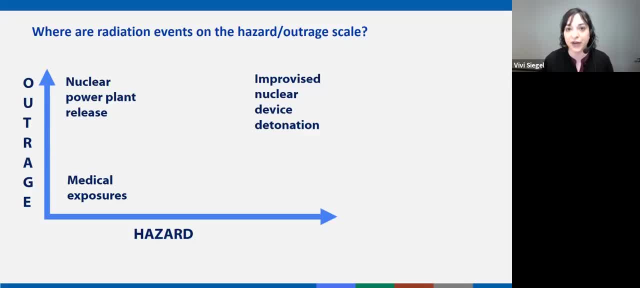 It's something that they're choosing to do for themselves, for their health. They know the risk-benefit relationship and they're making a conscious choice, Whereas something like a nuclear power plant release it may be a very low risk to the public. 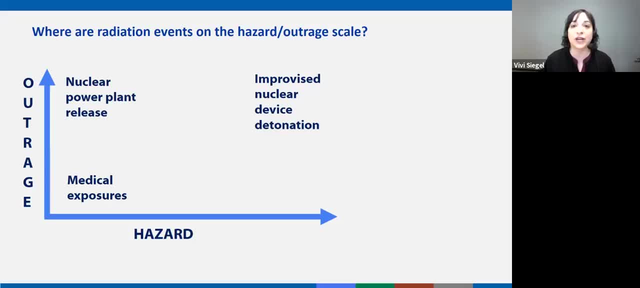 But the perception is a lot higher. outrage because it's something that people don't control for themselves. It is happening to them and it's being controlled by others And it's not a choice. So that's an example of something that may be low hazard, high outrage. 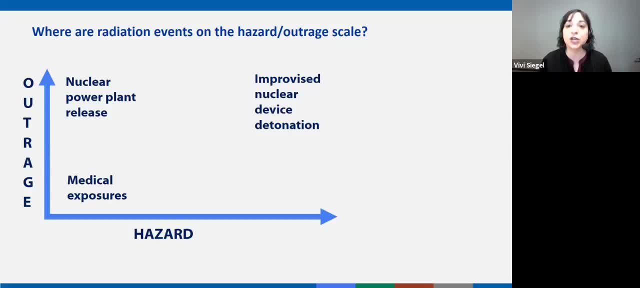 Whereas something like an improvised nuclear device detonation could be both high risk to people or high hazard and high outrage, because it's something that is happening that we didn't choose, that's being forced upon us And the situations where we're talking about high outrage events. 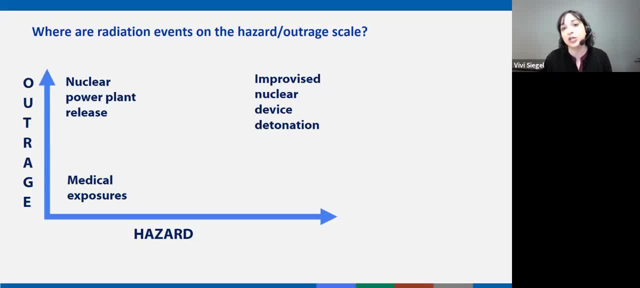 the CERC principles are more important than ever. Using empathy, speaking to people in clear, plain language that they can understand, giving people actions that they can take, can all help reduce the extra anxiety that comes from being angered and being outraged, as well as being in danger. 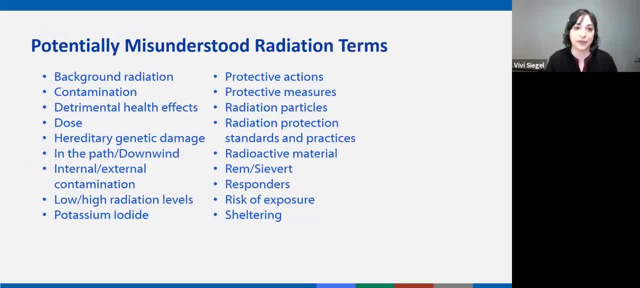 Next slide, please. I'm not going to define all of these for you, but I wanted to point out some of the terms that we have, And CDC has actually a radiation glossary on emergencycdcgov slash radiation where you can read about different radiation terms and find some plain language definitions. 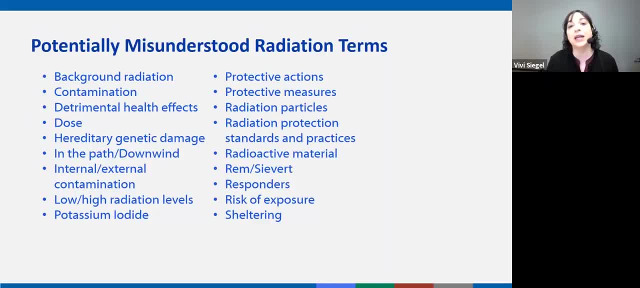 There are some things that would be ideas that people may not have heard about before, And we talk about things in a different way. For example, the word exposure means something different when we're talking about being exposed to an infectious disease versus being exposed to radiation. 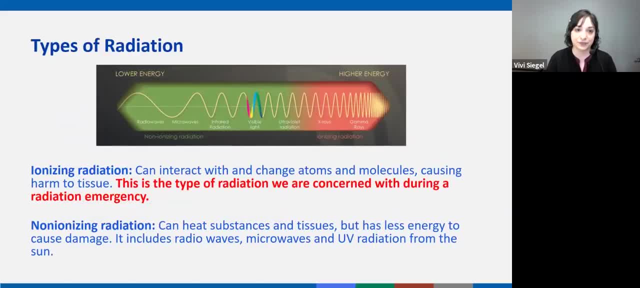 Next slide, please. Types of radiation. And again, this isn't meant to be a lesson in radiation, but I just wanted everyone watching and listening to be aware that there are different types of radiation: The type that, for example, comes from radio waves, microwaves, UV radiation. 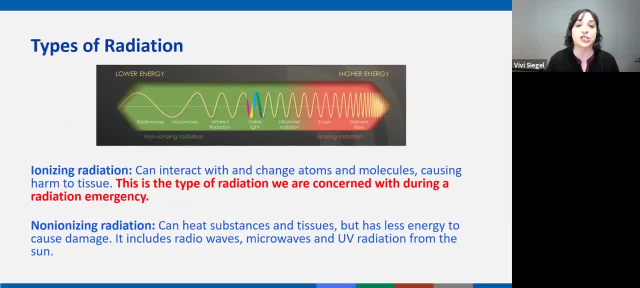 can cause anxiety, It can cause heat, but it doesn't change with or interact with our DNA. And the type that we're concerned about in a radiation emergency is ionizing radiation, because it can interact with and change molecules and that can cause health problems. 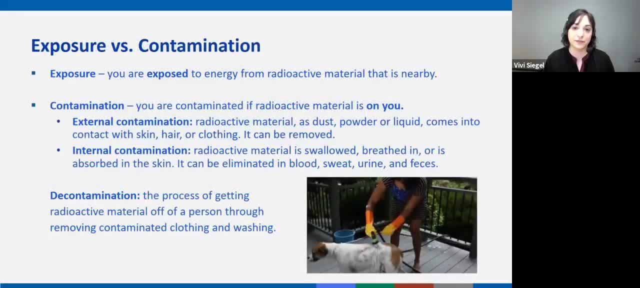 Next slide, please. So a little bit more about exposure versus contamination. So you're contaminated if there is some radioactive material on you, And this is something. that's a concept that's kind of difficult. It takes people a few times to really understand it. 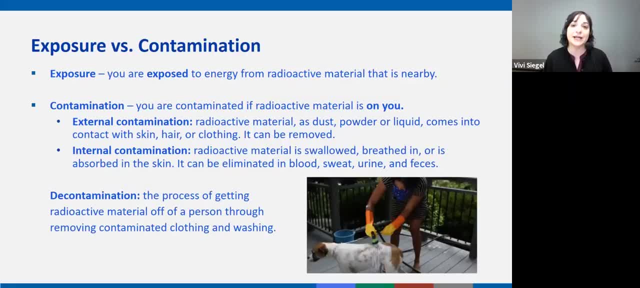 but you can actually wash off radioactive material as if it were dust. You can take a shower, You can take your clothes off if you're contaminated with radioactive material, and that will remove the source of radiation. That's different from exposure, which in a radiation sense. 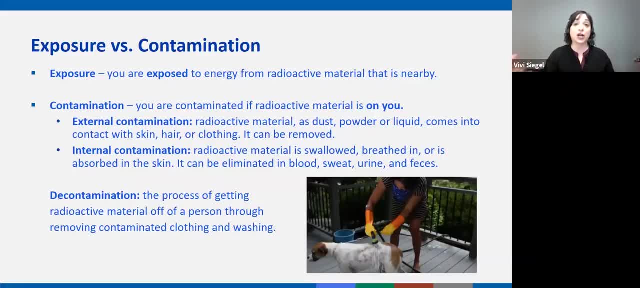 is that some of those energy waves are coming through our body and potentially could change our DNA. Now, of course, it all depends on dose- how much we're going to be affected by them, But exposure means you're being exposed to the radioactive energy. 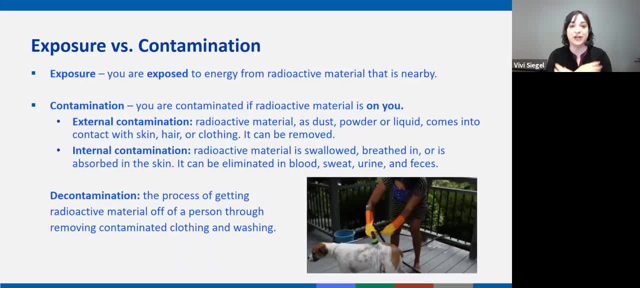 whereas contamination means you have particles of radiation on you that you can take off or wash off And you can be internally contaminated. Let's say you swallowed some radioactive material Or it's absorbed into your skin. You're contaminated internally. That can potentially cause some exposure. 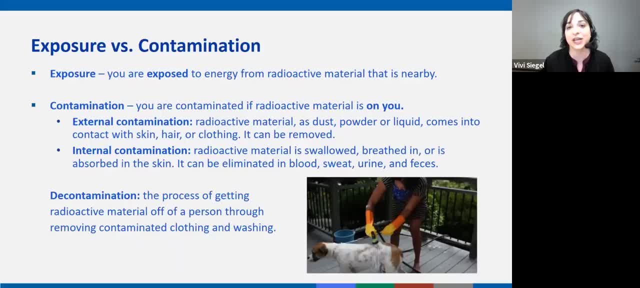 I know that's a little complicated and I'm sorry we don't have time to get into it here, but we do have some more in-depth trainings on the CDC website. if you're interested in learning more about that topic, If you go to emergencycdcgov, slash radiation. 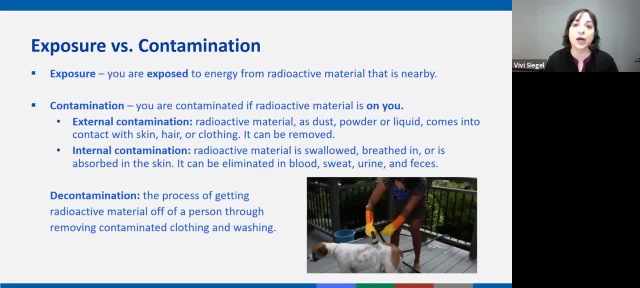 you can find a whole series on radiation basics, as well as more information about radiation communication, But I think the most important takeaway message for communicators here is that people should know that it's possible to decontaminate, As this person is doing here with the dog. 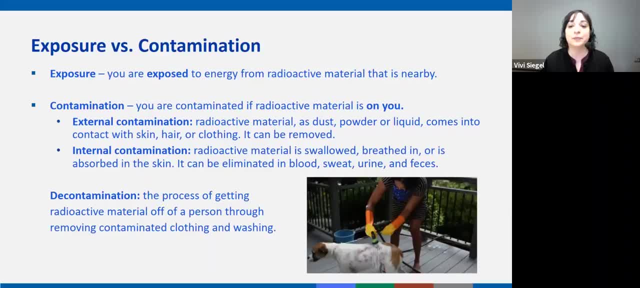 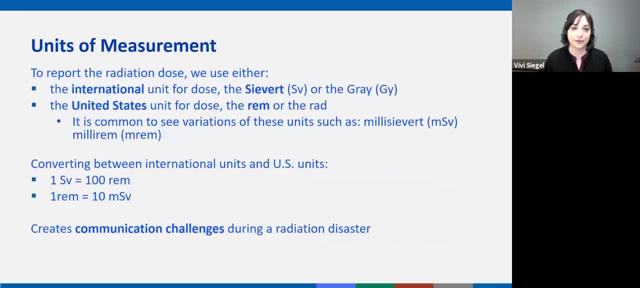 it's possible to decontaminate pets, too, by taking a shower and removing clothing. Next slide, please. Units of measurement are something that can also be really tricky to talk about, And I want to try to give you some examples. just to talk about a case where Haley said: 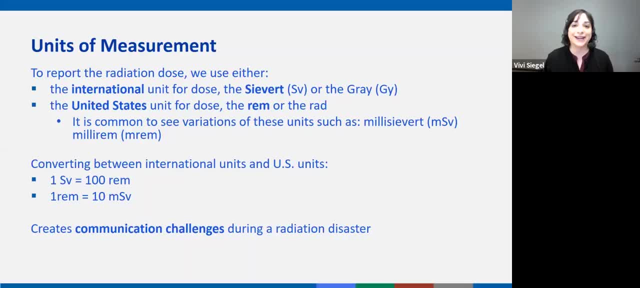 I was involved with a CDC response to the Japan Fukushima disaster And this was a case where it was an international situation and in the United States we use different units of measurement for radiation than are used internationally And this became a health communications issue. 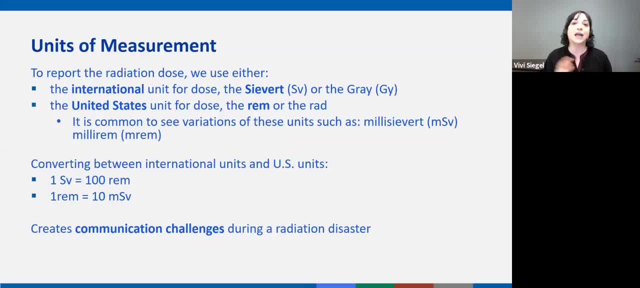 because not only did the scientists have to translate back and forth what units they're talking about to try to understand what doses of radiation people were being exposed to, but people listened to international news and people were hearing all kinds of numbers that weren't necessarily the numbers that we use in the United States. 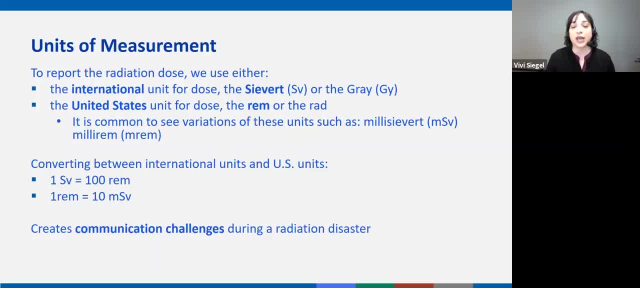 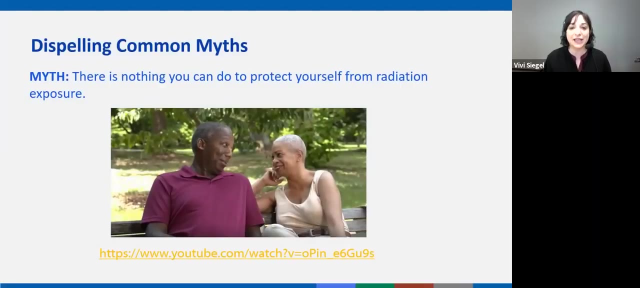 So it creates a language challenge and a communication challenge, and it's something we need to treat very carefully in the case of an international emergency. Next slide, please. Okay, so I'm going to talk a little bit about radiation myths And Haley, could you run the video? for this first myth is: 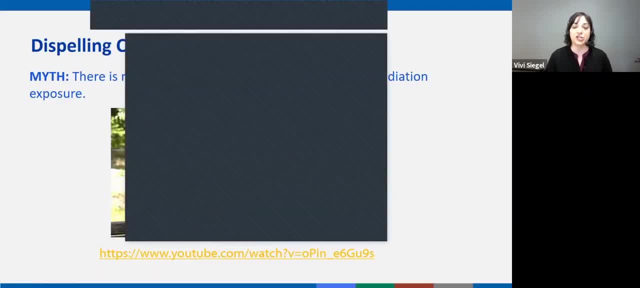 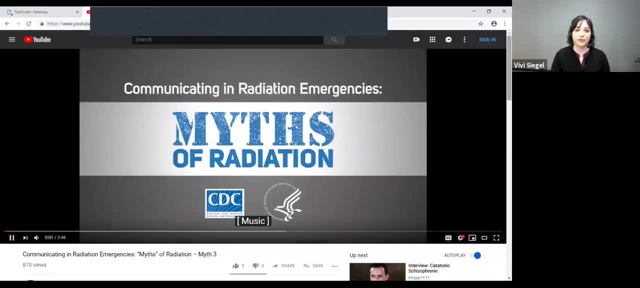 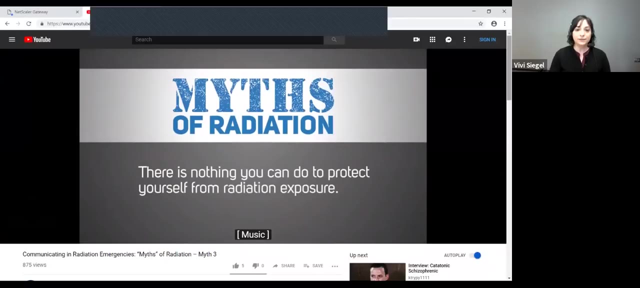 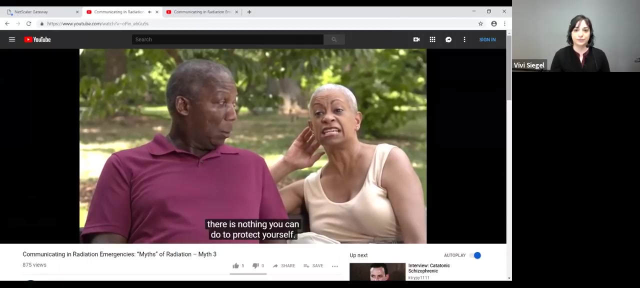 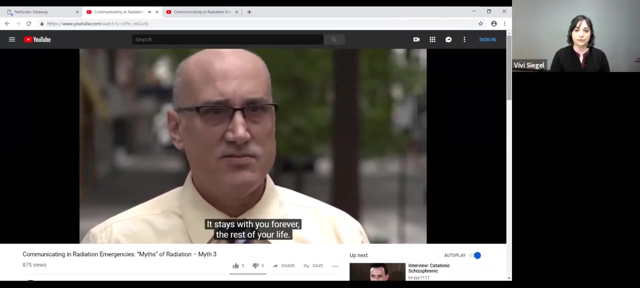 there's nothing you can do to protect yourself from radiation exposure, And we're going to watch about a 30-second long video. Radiation is scary because if you're being exposed, there's nothing you can do to protect yourself. Well, if radiation gets in you, it's there. 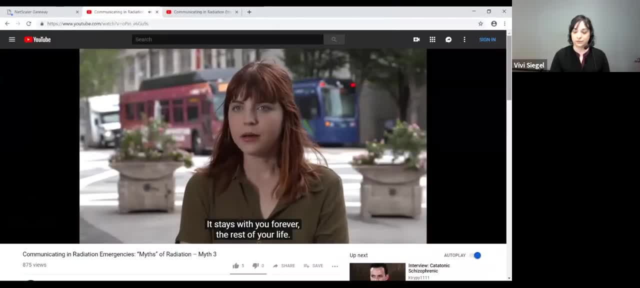 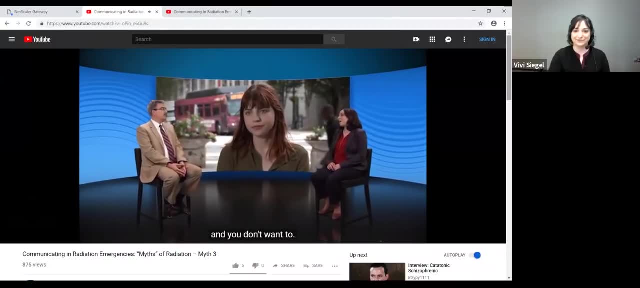 It stays with you forever, the rest of your life. Stay away from people with radiation, because you can get it from them and you don't want to Armin. these comments demonstrate that people feel more powerless when it comes to protecting themselves. 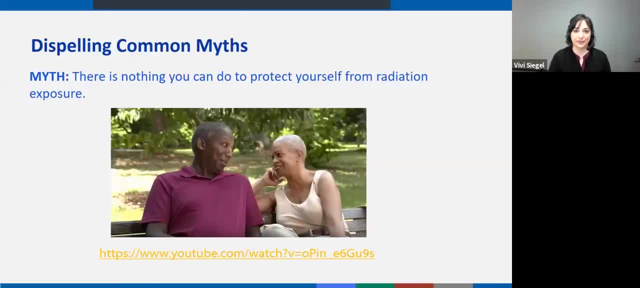 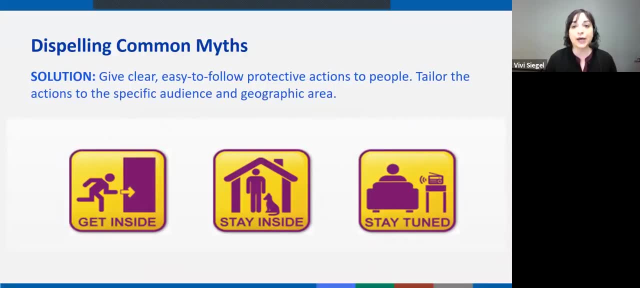 from radiation. So that is something that many people believe- that there's nothing you can do in the case of a radiation emergency, And so one of our biggest communication challenges is letting people know that not only are there things that you can do, but there are easy things you can do. 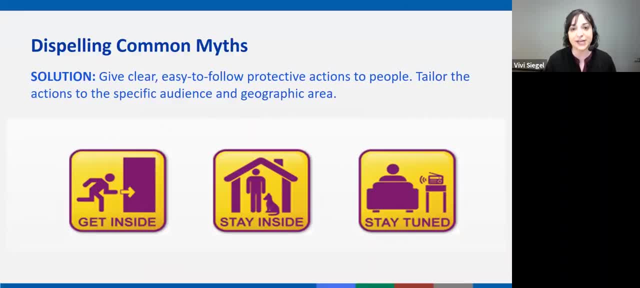 Our first message in a radiation emergency: get inside, stay inside and stay tuned. And this is something, a message that the US government has tested and adopted for its messaging that you'll see I'll talk about a little bit more further on. 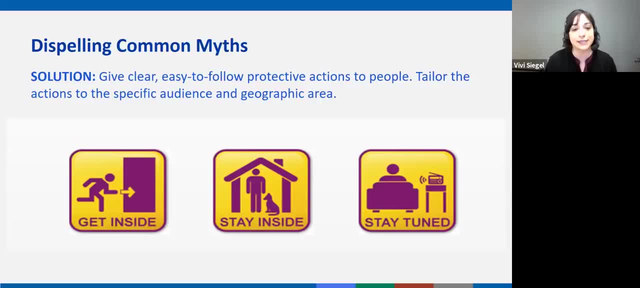 in the presentation, But get inside, stay inside and stay tuned. And the reason is because, as we were talking about, if there were a kind of nuclear explosion and nuclear energy is outside, actually putting a physical barrier between you and that energy. 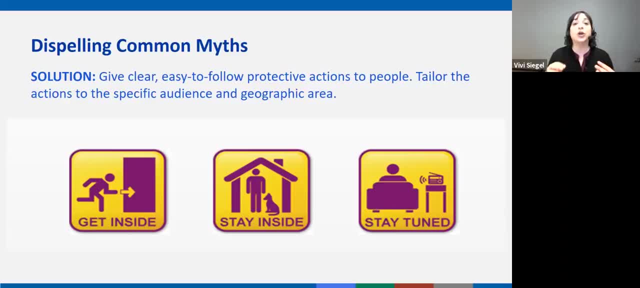 will protect you, And the farther inside you can go, the more protected you will be. So if you're in a house, you will be protected. If you're in a basement, you'll be more protected, And actually the taller the building is. 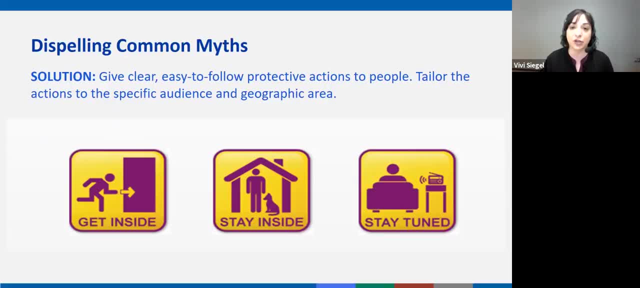 the more the bigger number of walls between you and the outside, the safer you'll be. And then our next message is to stay tuned. We know that certain types of biological particles have a half-life that will make them less powerful after a number of hours. 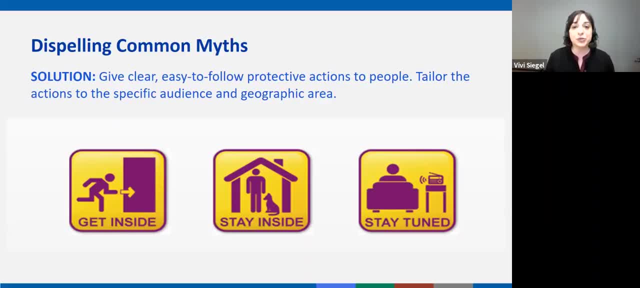 And so if you stay inside and stay tuned to the radio or instructions or emergency officials, you'll know when it's either safe to go outside to leave the area or safe to go outside and go about your business. So those are our major messages. 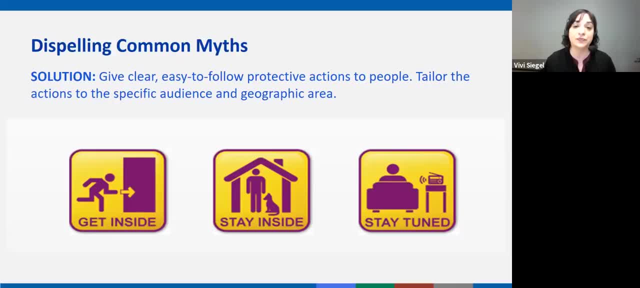 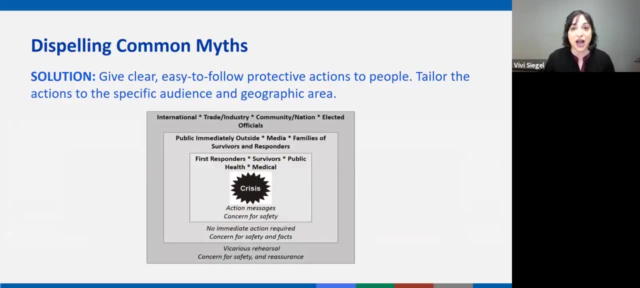 And if people know them, they'll do them. Then they won't know what to do. Next slide, please. We also believe in giving different protective actions to different people, depending on who they are- Obviously the people who are closest to the crisis. 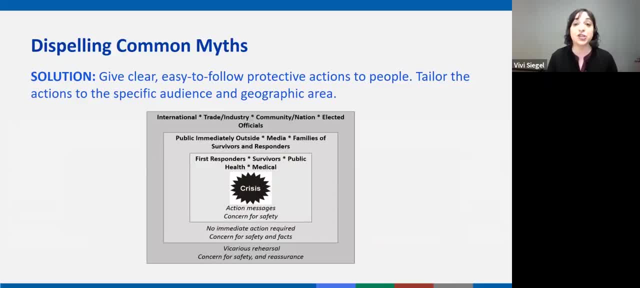 they need messages that will protect their safety. They need to know what to do to protect their lives and their safety. But people who are outside of the immediate crisis also need information: The media, the family, people who heard about it on the news. 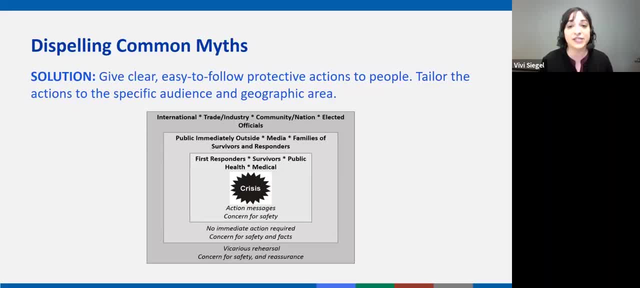 are worried about it, And we saw in the Fukushima disaster that in the United States we did not face any major threats to our health, but people were extremely worried about the potential for radiation coming across the Pacific Ocean from Japan And even though they weren't in any 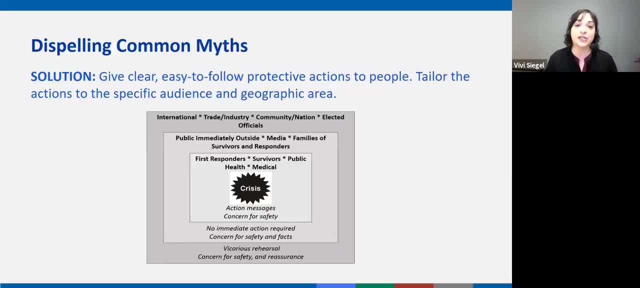 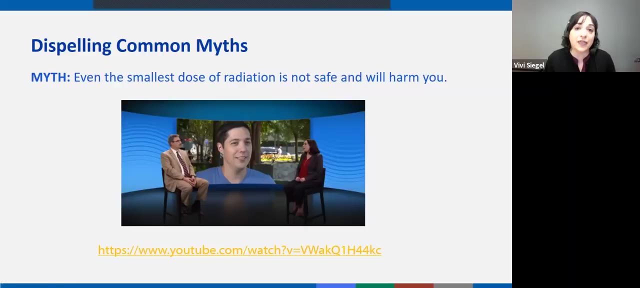 health danger. they needed information And they were looking for information, And so we need to provide tailored information to people in different circumstances depending on their circumstances. Next slide, please. Another myth that we hear often is about dose- That people don't believe that. 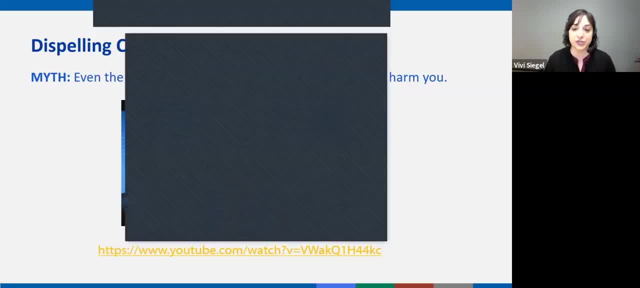 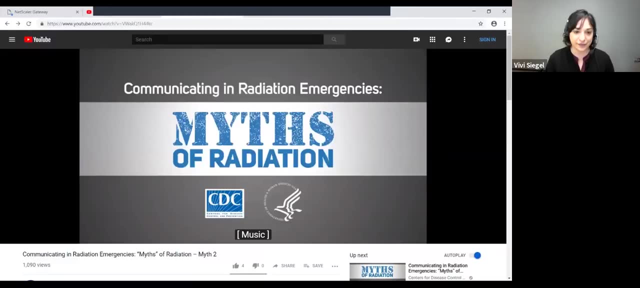 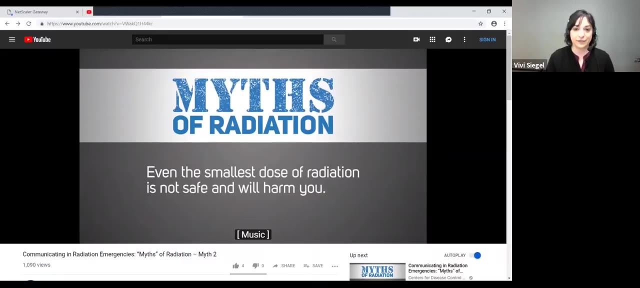 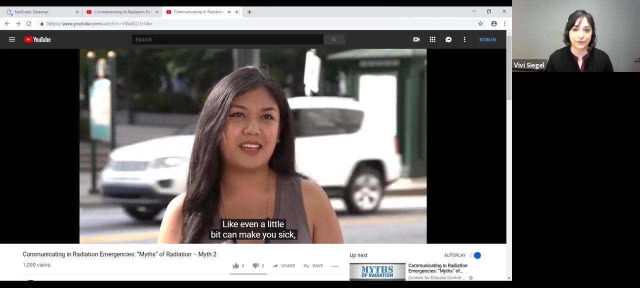 a small dose of radiation might not cause as much harm as a large dose, So let's listen in a little bit. Thanks, Hailey. No, I don't think it's ever safe to be around radiation Like even a little bit can make you sick. 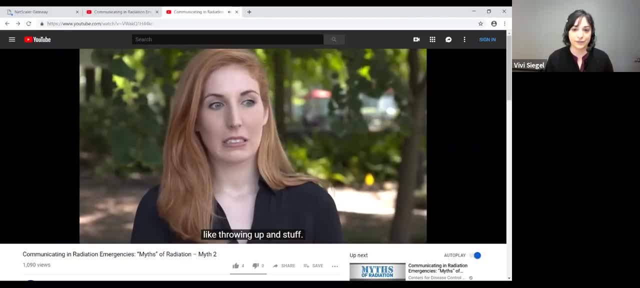 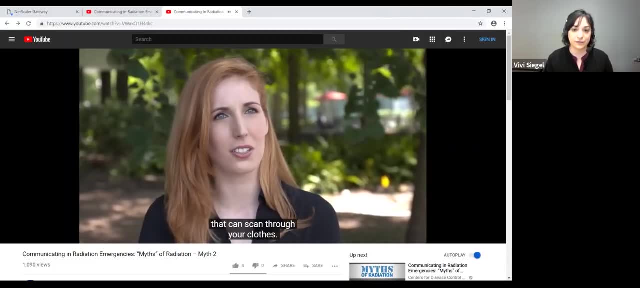 Like throwing up and stuff, Um, I don't know. Any kind of radiation is dangerous. I mean, that's why they took those machines out of the airports, The ones that can scan through your clothes. It was too much radiation for people to be around. 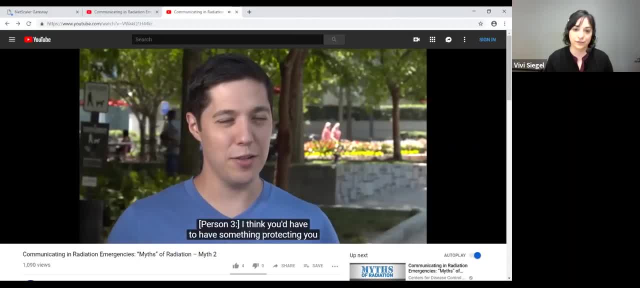 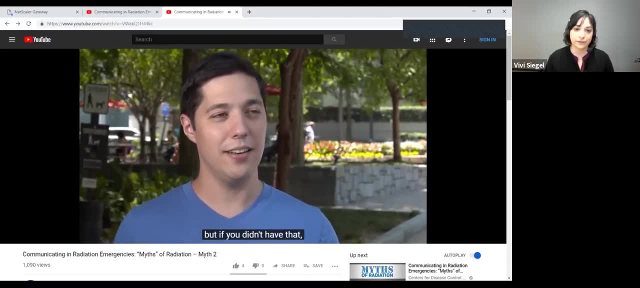 It could have made someone sick. I think you'd have to have something protecting you. Like what's the thing at the doctor's, like the lead thing they put in front of you for an x-ray? I don't know that. I think that it's definitely not safe. 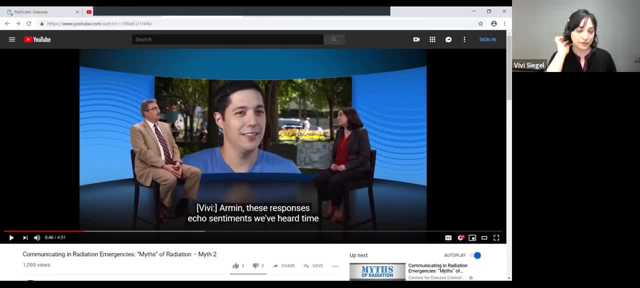 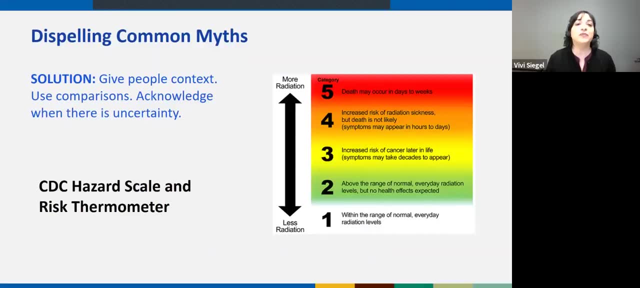 Thank you, Hailey. So what do we do if people think that any amount of radiation is the same? We try to give people context, And in risk communication it can be a little tricky to use comparisons, And those of you who are communicators- 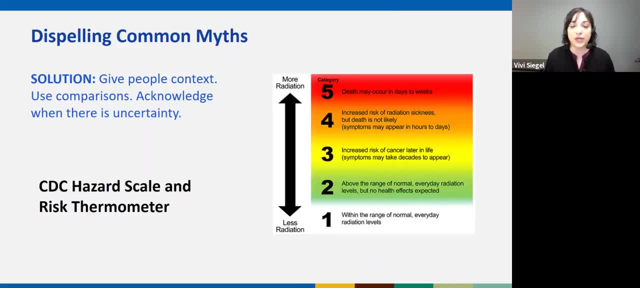 are probably nodding as I say this. you may have had some instances where it didn't work out well when you're comparing one risk to another, Particularly a risk that is voluntary versus an involuntary risk. But we found that people just have no context when it comes to radiation. 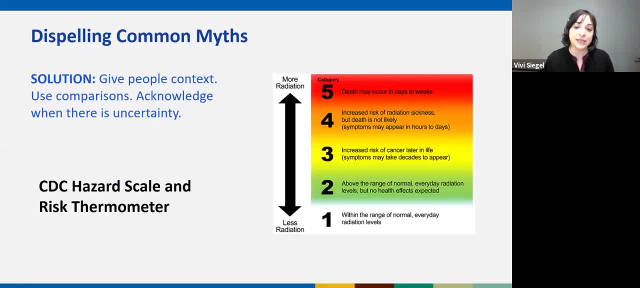 that it can be helpful to share with them some of the that they're exposed to radiation every day and that some radiation falls within normal everyday radiation levels. So this is a thermometer, a hazard scale. I'm going to show you the hazard scale. 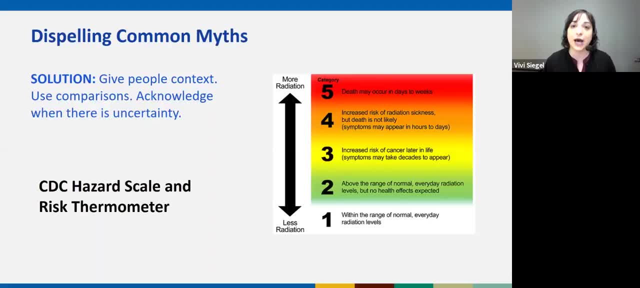 and the thermometer that CDC developed, spoke with focus groups and audiences and has been sharing this with partners as a way to share with people the different levels of risk of radiation that they might face. So, as you can see, in this hazard scale, category 5 is extremely dangerous. 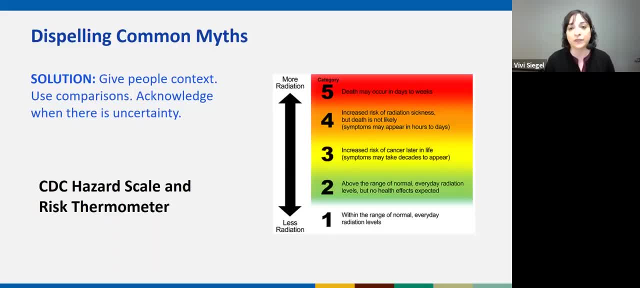 whereas it goes down to category 1, which is within the range of normal everyday radiation, And it could be used in instances where we're talking about: well you know, if you're outside and you're being exposed to the energy that's outside, you may be at a category 3. 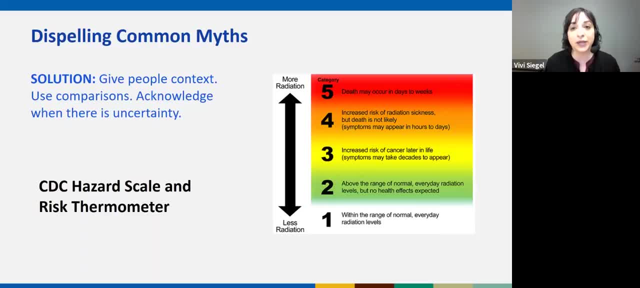 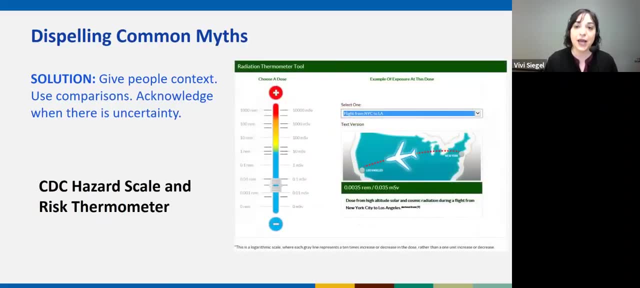 but if you go inside, you could reduce that to a category 2 or 1.. So, in helping people make educated decisions about their own safety, Next slide, please. And then this is an interactive radiation thermometer tool you can find on our website and you can actually. 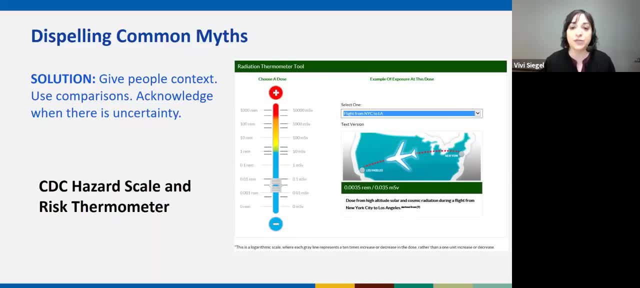 click and you can slide this bar up and down to choose the rems or sieverts that you're exposed to and it will give you an example of an exposure at that dose. So, for example, this is saying that a cross country flight would be equal to: 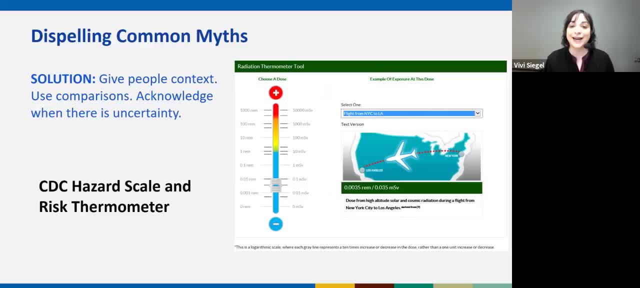 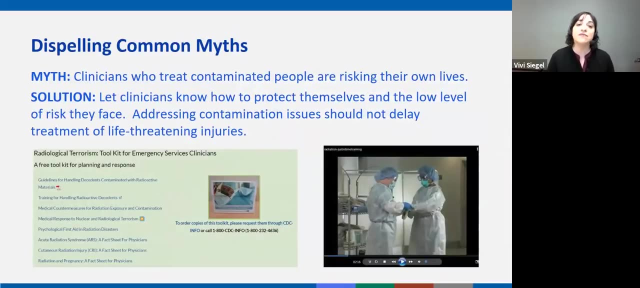 this dose So people can see what's a more everyday level of exposure and what leads to a more dangerous level of exposure. Next slide, please. We have another myth that is very common. I don't have a video for this, but because of the fear surrounding. 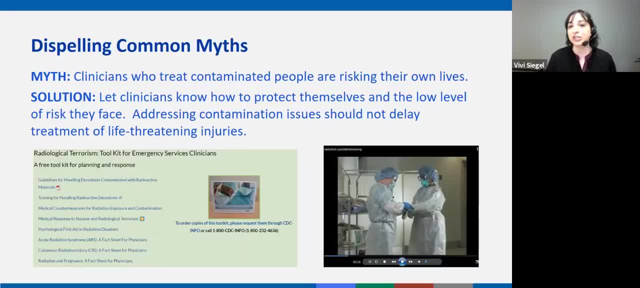 radiation exposure. medical professionals are scared too. Emergency responders are scared too. They don't know if it's safe to go and help people. They don't know if people are coming to the hospital is it safe to treat them. So we're working to educate. 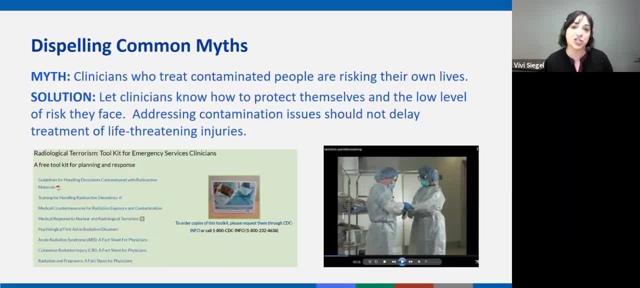 medical professionals as well and have some tools and information on our website, and that we can send a toolkit for medical professionals to share with them. that you can treat people who have been decontaminated for issues that they might have They might come in with. 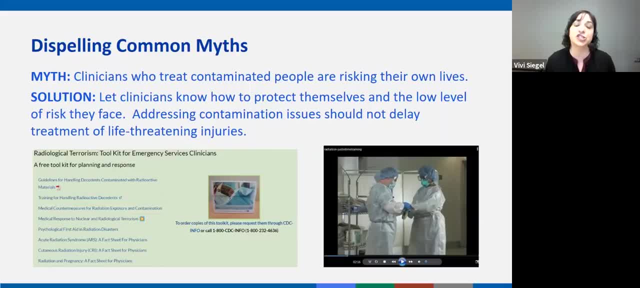 some trauma issues that they need to see a doctor for, and physicians should not be afraid to treat them because of fears for their own safety. So these tools that we have on the website can help medical professionals understand what's a risk and what's not, and how they can protect themselves. 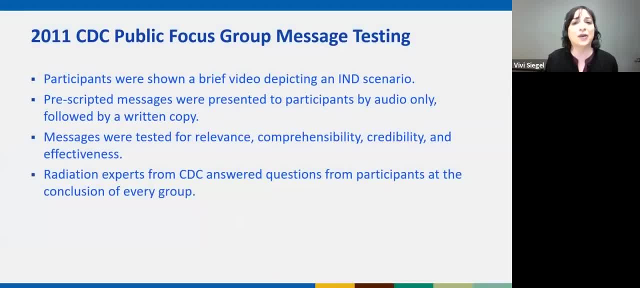 Next slide, please. Okay, so what do we know about radiation messaging so far? I'm going to go back a few years to some message testing that CDC has done, and CDC has been working with our partners on message testing for about the past decade- or a little longer to see. 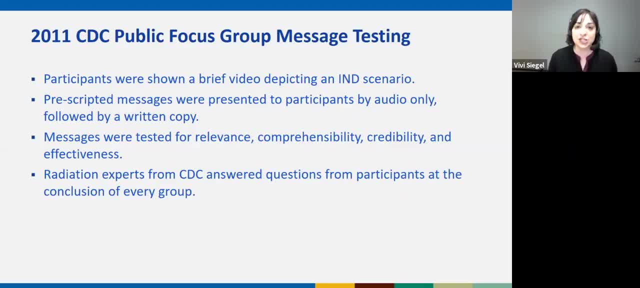 what messages resonate with people, and we're still working on new messages, and this is something that we're constantly trying to improve on and work on. But this was message testing about an improvised nuclear device scenario- so about a nuclear explosion- and we tested them and then we got feedback. 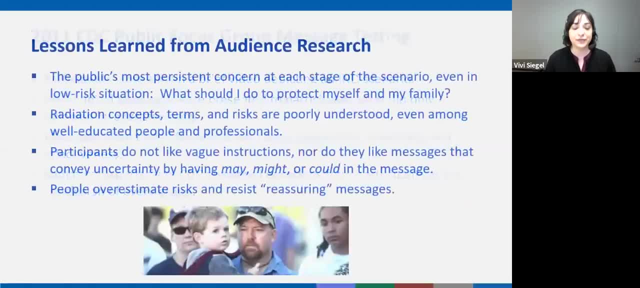 So go ahead to the next slide, please. As you might expect, the most prevalent and persistent concern is: how do I protect myself? How do I protect my family? Radiation concepts and terms are very poorly understood even by very well educated people, Even if 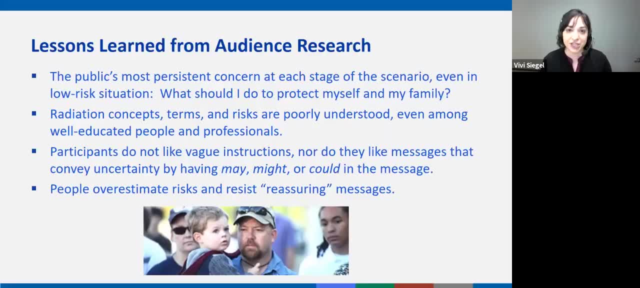 you have a PhD. if it's not in radiation, you might need some information in plain language, and I know that you probably already know this, but in an emergency, our comprehension level really falls When we're worried about: are we safe, Is our family safe? 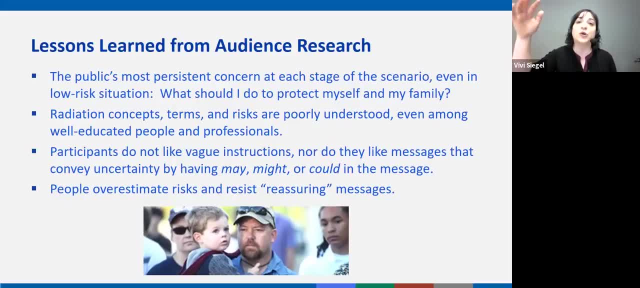 I may be able to understand grade 12 information on a normal day, but I might need grade 3,, grade 4, grade 5 information on a day when I'm really anxious and worried about my kids. People don't like uncertainty. Well, some of that is unavoidable. 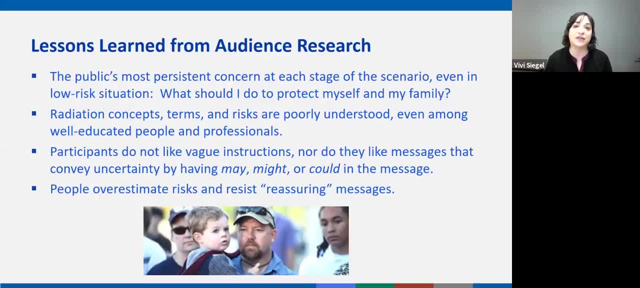 we are not going to have all of the answers. we will have uncertainty, but we need to recognize that it's going to be an uncomfortable message and help people as much as possible by talking about what the process is to learn more information And people will overestimate. 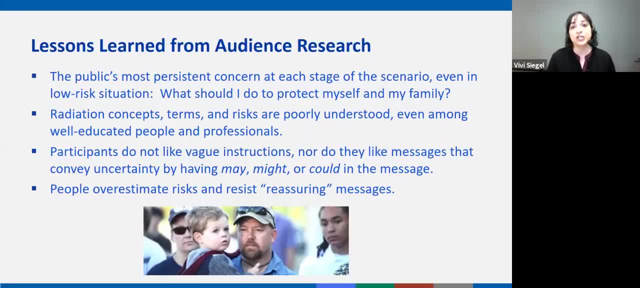 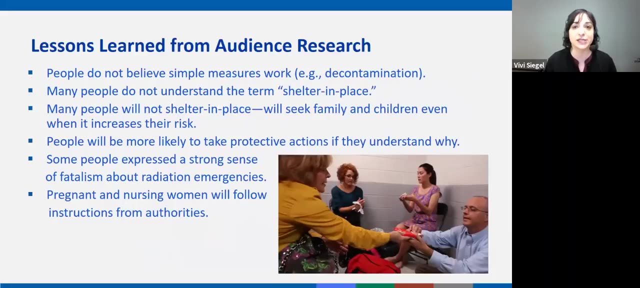 risks and resist reassuring messages. They don't want to hear: you're fine, you're safe. They want to hear what the specific risk is and what they need to do. Next slide, please. They don't believe decontamination works. It's something that we still need to do. 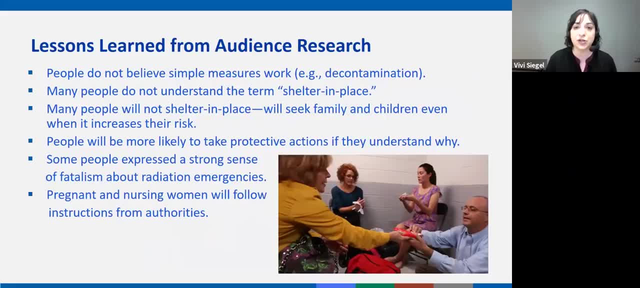 a lot of education about. They don't understand shelter in place or go inside, stay inside and stay tuned, And this is something that really resonates with me. as a mother of two small children, I know that if something like this were to happen- and I was at work- 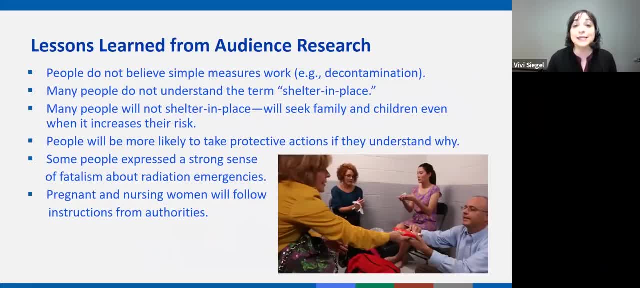 and my kids were at daycare, my immediate instinct would be to try to get to them as soon as possible. A lot of people share that instinct, where they want to go make sure their families are safe and they don't want to stay, Whereas the safest thing to do is for me. 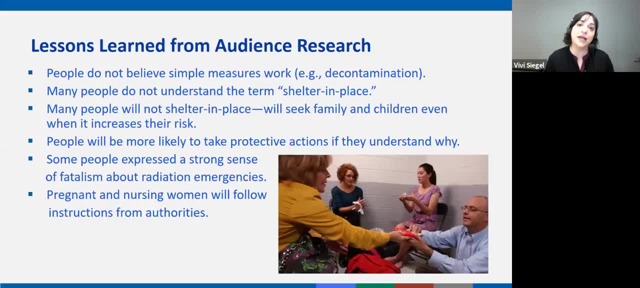 to shelter in place at work and for them to shelter in place at their daycare, And so we need to not only get the message out that that's the safest thing and that leaving could put us in danger, but also that schools and daycares and places of work have measures in place. 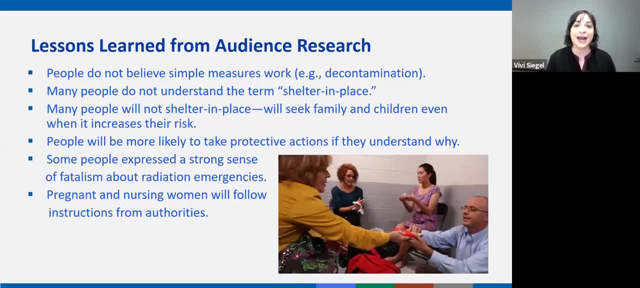 for this and other types of emergencies to keep people safe, And so we know if we can just wait 24 hours or so that we'll be able to reunite again. People will be more likely to do this if they understand why or if they understand the risks involved. 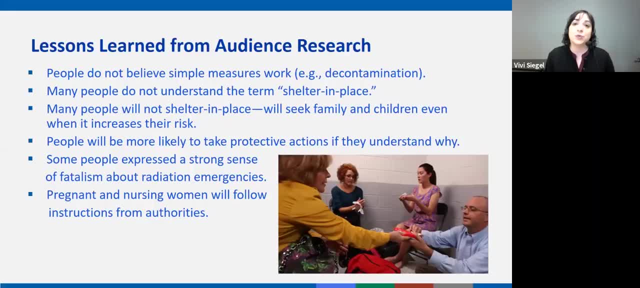 and how much sheltering in place will protect them. And we found that people who are pregnant or nursing are more open to listening to instructions from authorities and they're looking for information. so we need to be prepared with that information and have it ready for them. 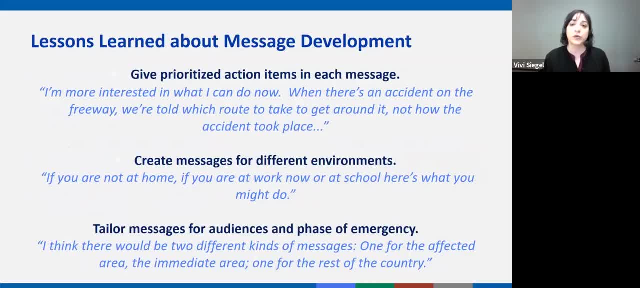 Next slide, please, And here's just some quotes from people from the focus groups. They want to know. you know what do I do? What do I need to do to protect myself? We need to tailor messages for audiences. different phases of the emergency. 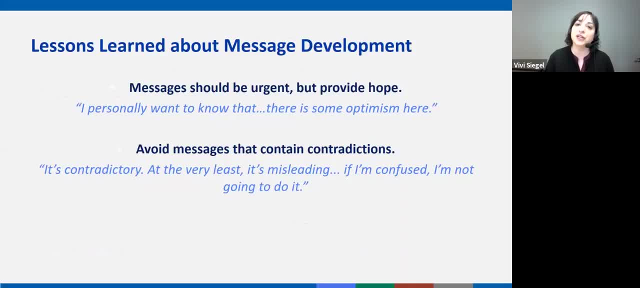 And we need to be very careful with what we're saying and what we're saying to the audience. This can be really difficult, especially if there are a lot of different entities responding to an event And since you work in emergency response, I'm sure you've been in this situation. 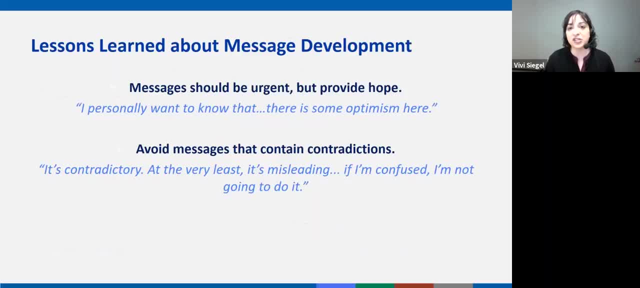 where there are. there's a lot going on and people might be hearing information from different sources, So that's why it's so important to coordinate with all of the responding agencies to follow the structures that are in place to make sure that we're getting the right. 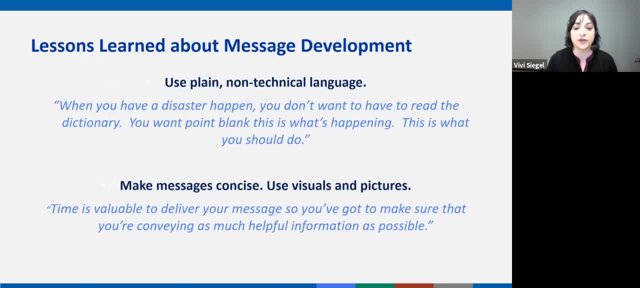 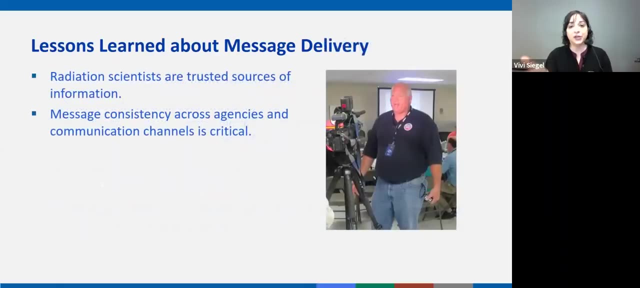 communication message And seeing a question about tools that we use for audience research. you can find a more in-depth report about our audience testing and audience research on the website emergencycdcgov, and the links are coming up. Next slide please, And using plain, non-technical language. 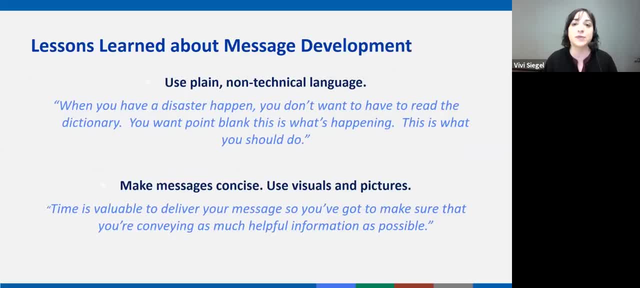 and visuals and pictures wherever possible. We've actually developed a series of infographics to help with communicating about the information that we use, And we have a number of infographics that are available on our website and they've been adopted internationally, some of them for use. 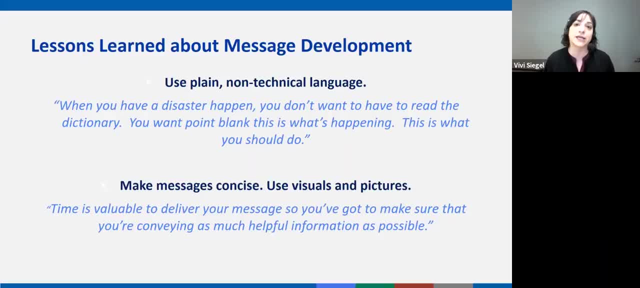 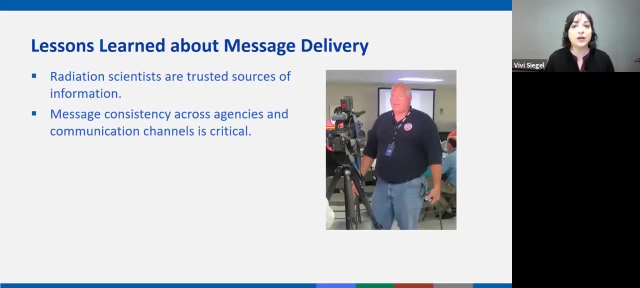 And, of course, we're always looking for more tested ways to share information and easy to understand visual manner. Next slide, please. Finally, we know that who delivers the information is just as important as what they're saying. Are they using empathy? Is it someone? 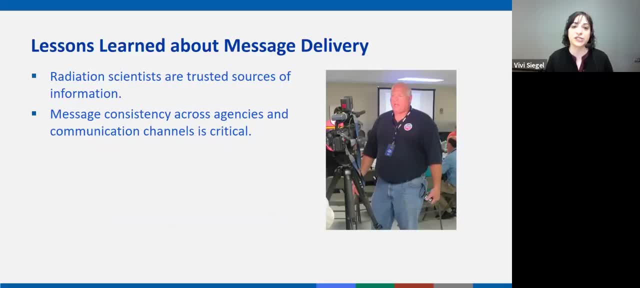 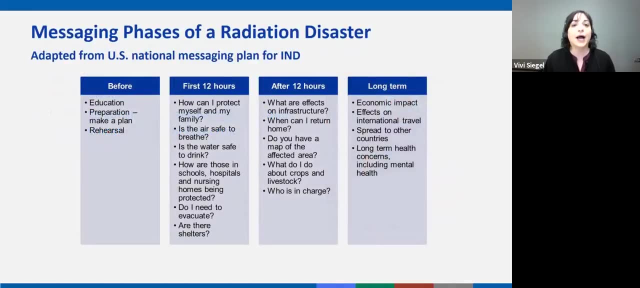 with a critical level of authority. Is it someone who can be trusted? And again, consistency is critical. Next slide, please. I just wanted to share that. just like in a natural disaster, when we're talking about the different phases, say, of a hurricane response, there are different things. 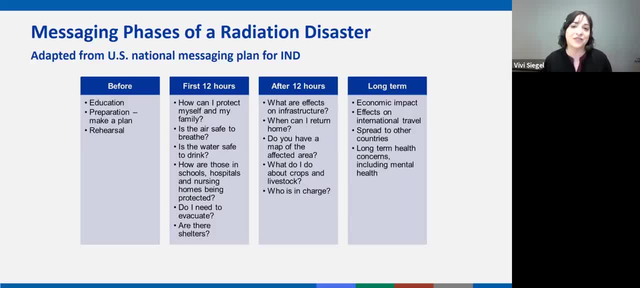 that we know are going to come up. different questions we know people will have before the hurricane, during the hurricane, after the hurricane. we can anticipate those questions and we can be prepared with messaging for the things that we know. Obviously every event is unique and there will be some things. 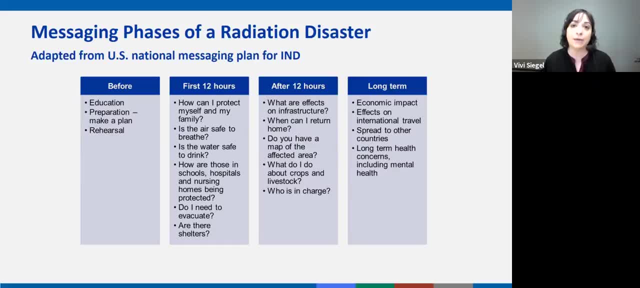 that come up that we might not have thought about before. but many of the questions are predictable And same with a radiation disaster and the US National Messaging Plan has divided things out into the first 12 hours and after the first 12 hours, and I've divided this out a little bit. 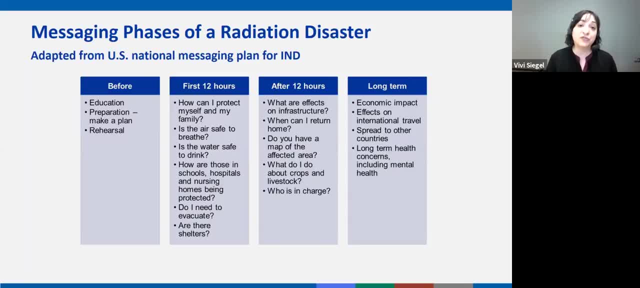 before, to talk about what we can do before something like this ever happens. How can we prepare, How can we educate, How can we rehearse? And then, long term, we know that the issues are, the questions don't go away for years and years. We see it in: 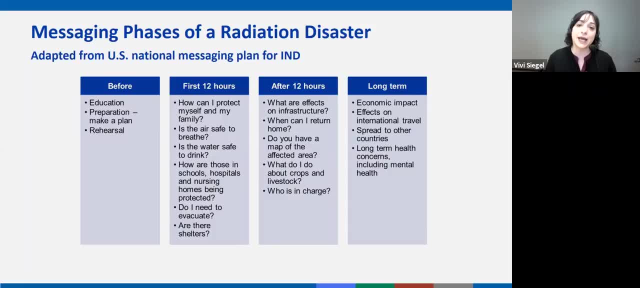 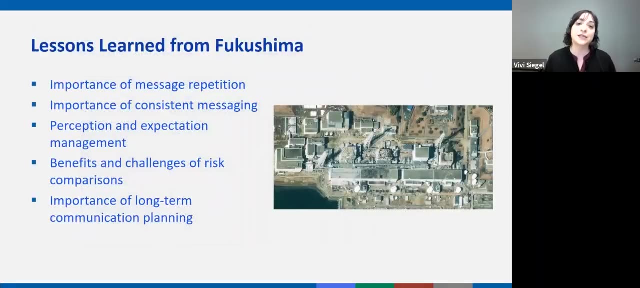 Chernobyl. we see it in Fukushima. we see it in cases that have happened here, where, even though the immediate threat is gone, the questions remain. Next slide, please. So, speaking of Fukushima, some lessons that we've learned, consistency, and I just want to highlight the last bullet. 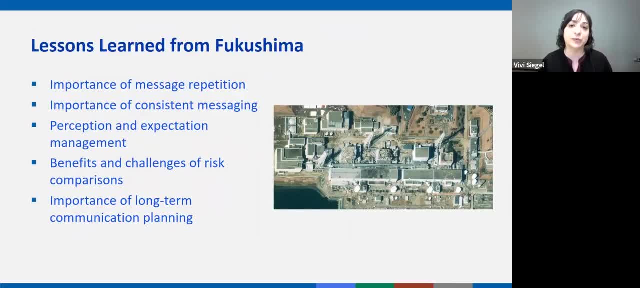 here the importance of long term communication planning. Not only, what are we going to say right after a disaster, but do we have communications infrastructure in place to keep information coming to a community that's going to need it for many years? And the questions that are going to continue. 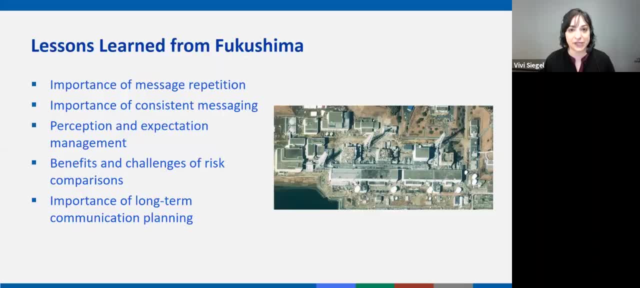 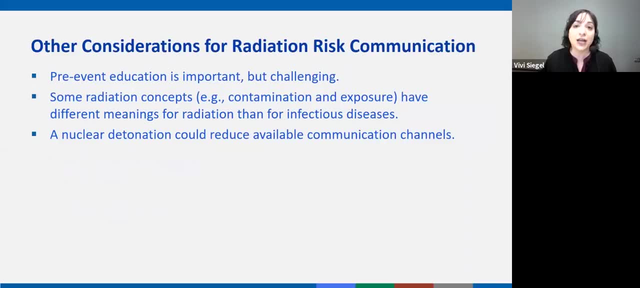 to arise. Next slide, please. So this can be really challenging to do, Especially talking about radiation risks when there aren't any imminent radiation risks. It's not a comfortable topic to talk about. It's not anything that people like to think about. 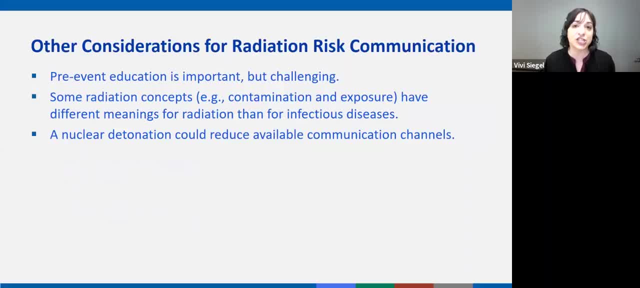 I know I certainly don't, So it's a challenging thing and it's something that we're working on, and I know many of our public health partners are also working on. what are the best ways to get information to people so that they can be prepared. 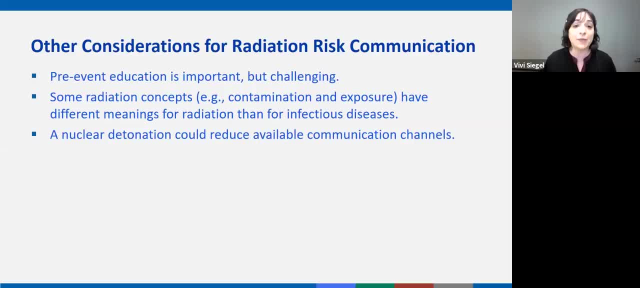 but not scared but ready in the case that something like this might happen. We also know that this is like I said before. radiation is a different beast than infectious disease. It might not be something that the people who are well practiced in risk comm for infectious 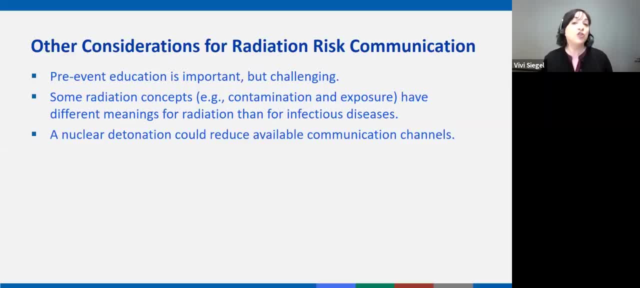 diseases are ready to take on radiation, so there may be some cross training that needs to happen at different levels of an organization. And finally- and I know Jonathan Lynch on the EPIC team, sitting next to me, knows a lot about this nuclear detonation- 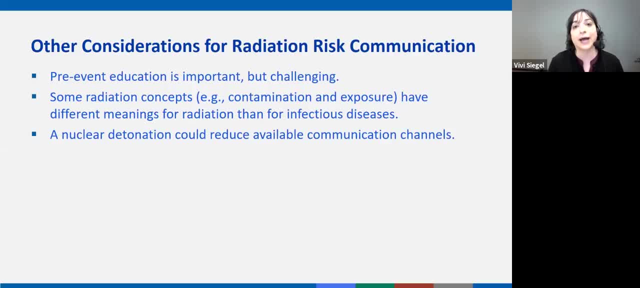 could reduce available communication channels And we might not have social media, broadcast media, immediately available to us. We might not be able to reach people who most need the messages. So what are the things that we can do to have other backup measures in place? 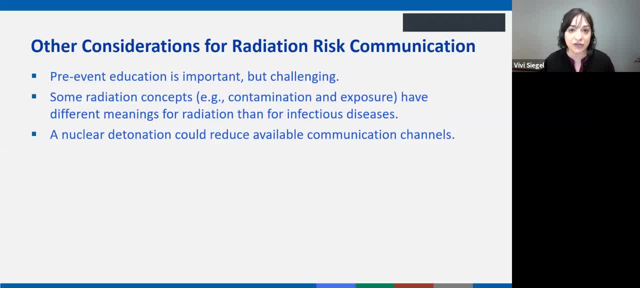 And we need to have them not only on a federal level, but at the local level. Do you know what your backup communications capabilities are And what are the ways that we can get information to people before they need it, so that they have it and they're ready? 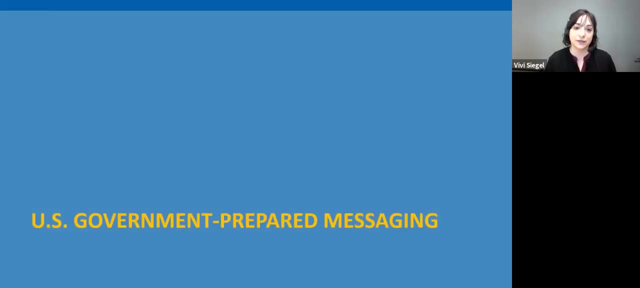 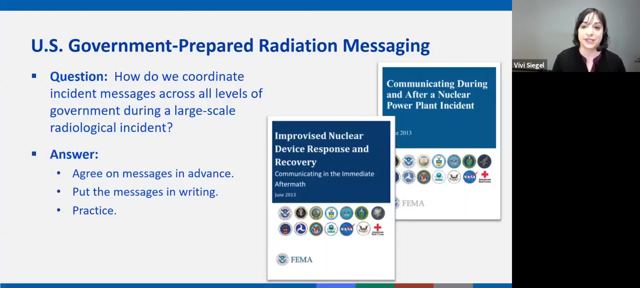 Next slide, please. So what has CDC done and what has the government done so far about these types of messaging? So you see here a couple of documents that were released in 2013 after several years of collaboration and message testing, and all of the agencies whose 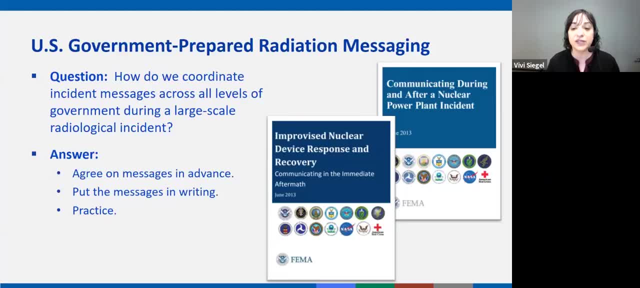 logos you see on the documents were included and involved in this process led by FEMA, And we know that one thing we can do to make sure we're all ready is to talk about it, To agree on messages in advance, put the messages in writing and then practice, And so 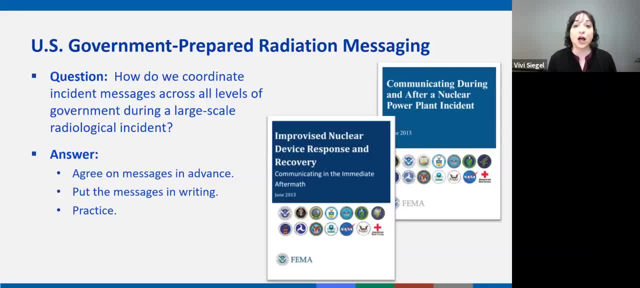 Haley mentioned, the 2017 Gotham Shield exercise is one way that the federal government has practiced these types of scenarios, So hopefully they're not something that we'll ever have to do in real life, But if it does, it won't be the first time we've thought about it. 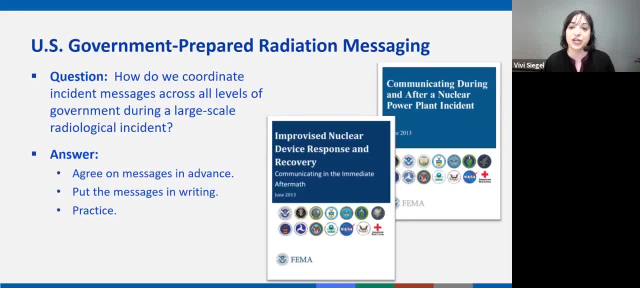 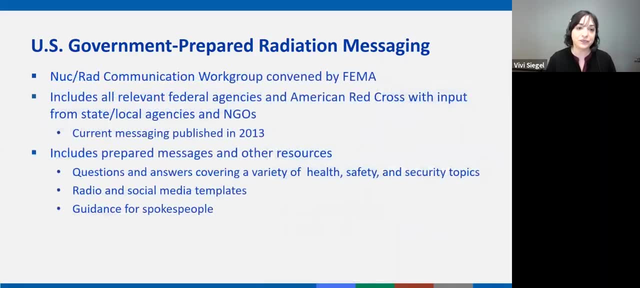 And there's another document for communicating after a nuclear power plant release, And these documents have inside of them sample messages And next slide please. So there's prepared messages, Q&As, radio social media templates, guidance for spokespeople. 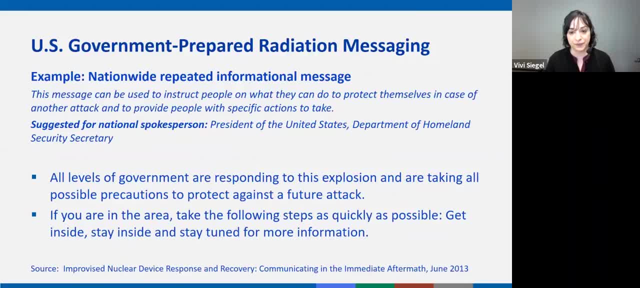 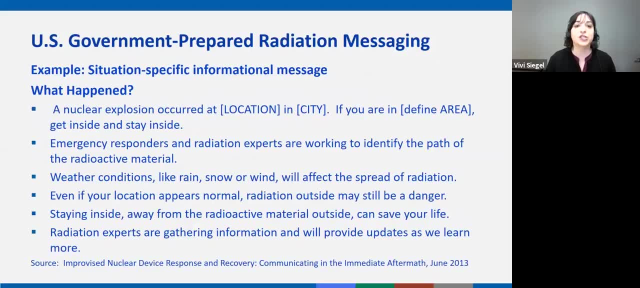 And here's an example of some of the messages that are in there. And so, like all other federal agencies, CDC participates in the national response plan and we follow- Oh, thank you, Jonathan, We follow- federal guidelines for how we would respond and what our role is. 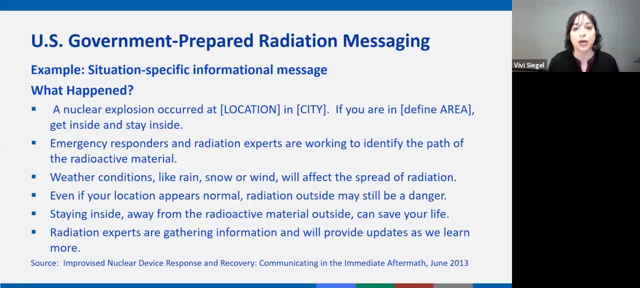 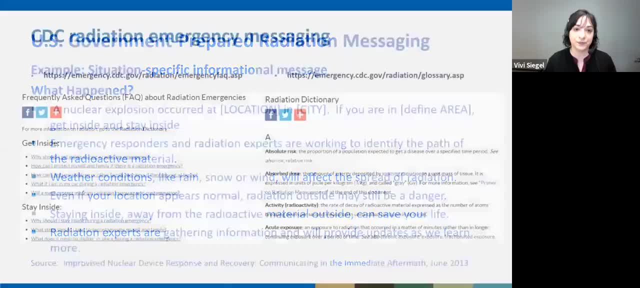 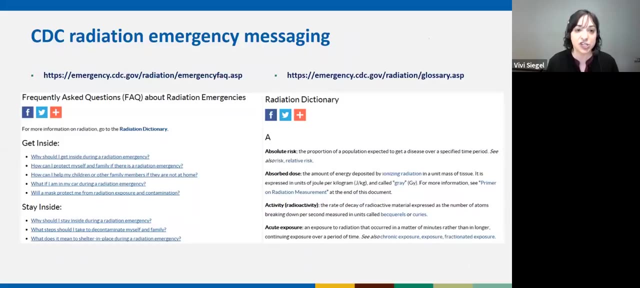 And we are certainly one small part of a very large, what would be a very large response if this were to happen? Next part, please. We also have radiation emergency messaging. that is on our website, As I mentioned, it's emergencycdcgov. 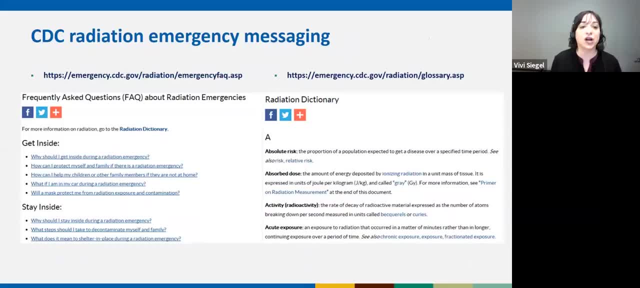 slash radiation And you can find our FAQ, answer some of these questions and our attempt at putting some of these difficult definitions in plain language. Obviously, we can always do better and it's something that we're working on, No matter how plain you think you are being. 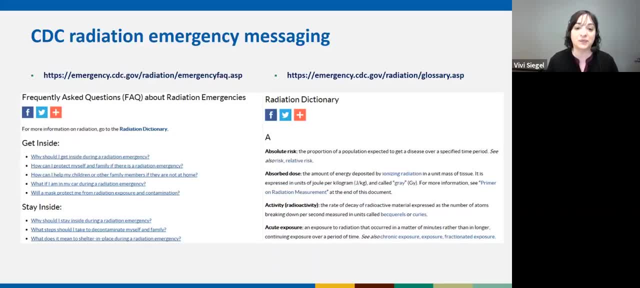 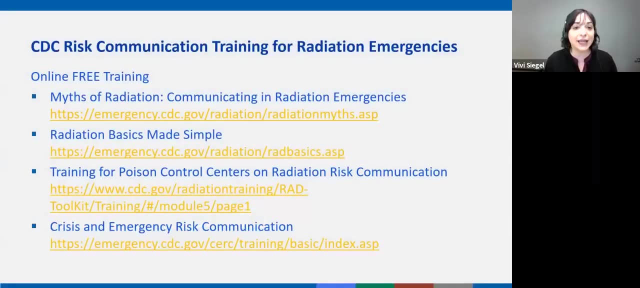 you can do better And so, but this was a pretty comprehensive radiation dictionary that we hope can help our partners get started or to learn about these terms. Next slide, please. Finally, like I said before, we have some trainings online. 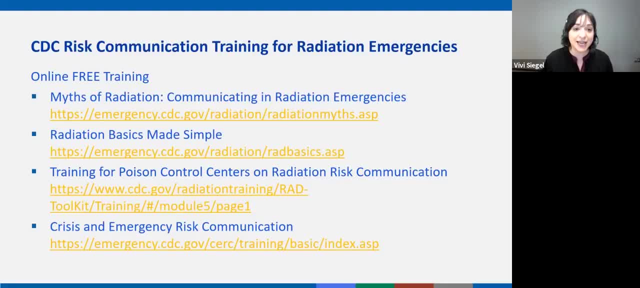 If you want to see the full myths presentation, it's at that first link. There's also the radiation basics presentation I spoke about. that will go a little bit more in depth about what is radiation and how to talk about it. We have a risk. 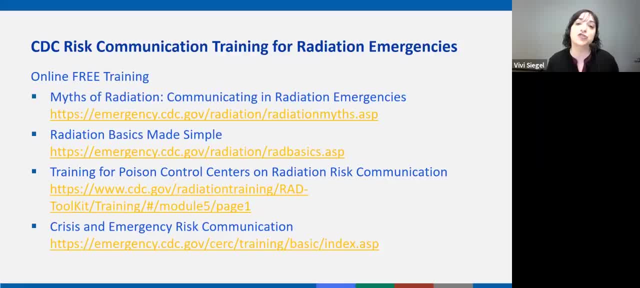 communication presentation that was designed for poison control centers, but it's actually pretty useful for anyone who might be getting questions about radiation and might be in the position of answering health questions. We have an online version of our full crisis and emergency risk communication training. 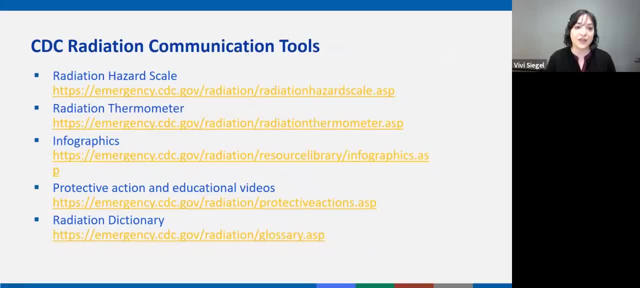 Next slide. And then here are some of the tools: the hazard scale, the thermometer infographics, the dictionary and, finally, some videos that show what protective actions look like and how people can take them. For those of you who are interested in learning more about our 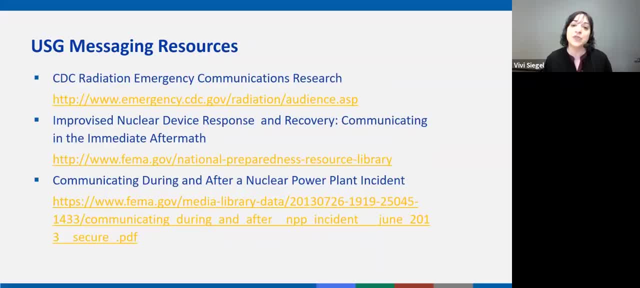 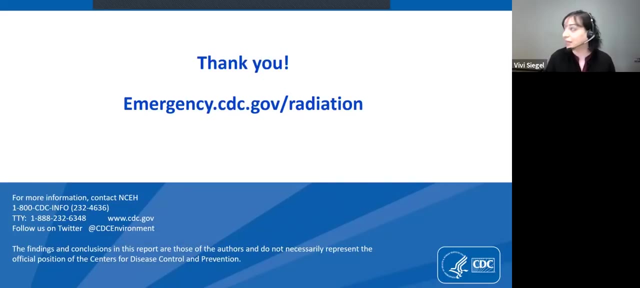 message testing and research. the top link there goes into greater depth about how those focus groups were conducted and the findings, And then below that are the two federal documents that I mentioned earlier. Thank you very much. Thank you to Haley and Jonathan and the. 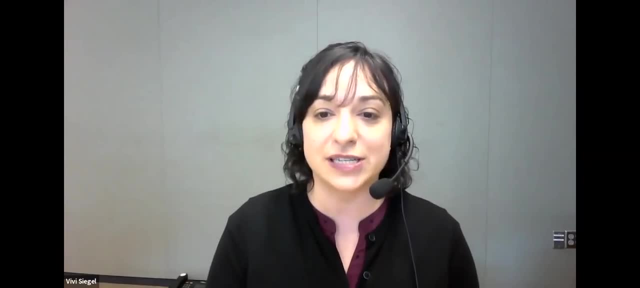 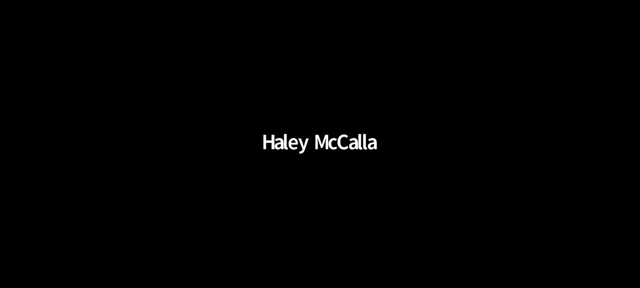 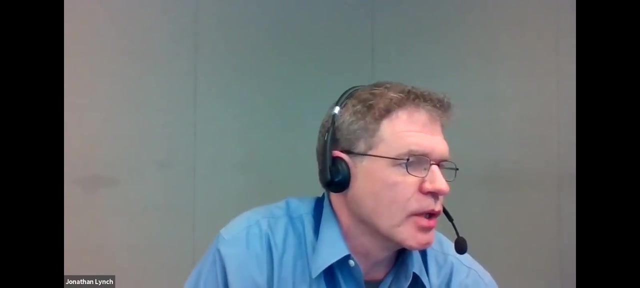 EPIC team for having me and I'd be happy to answer any questions now. We will now transition into the Q&A session. Jonathan, do we have our first question? Hi, yes, we do. Our first comment actually came early on from. 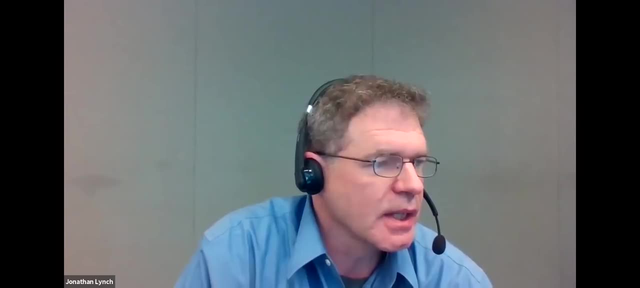 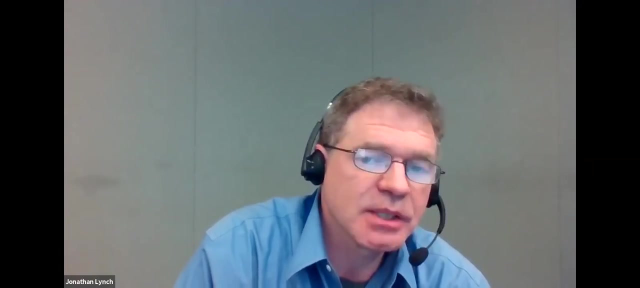 John Rice. He's from FEMA Region 1. He said I am in the Radiological Emergency Preparedness Program. We deal with the offsite response to incidents at a commercial nuclear power plant. I evaluate a lot of JIC slash JIS systems. JIC refers. 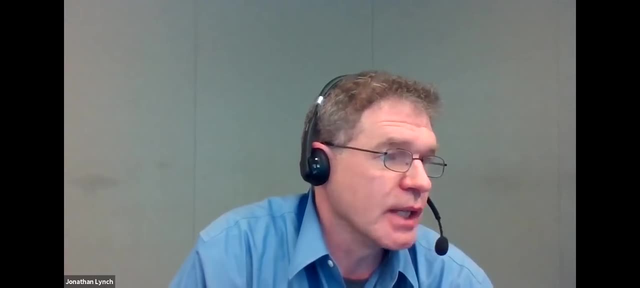 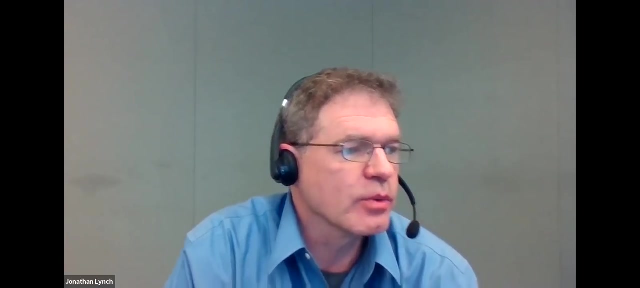 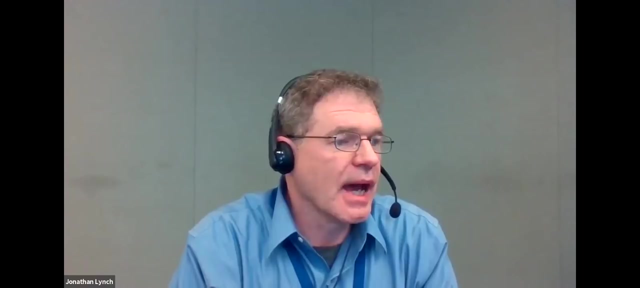 to a joint information center. My concern- and it was magnified during the Southern Exposure Exercise of 2015, is the lack of knowledge within the federal family of public information officers when it comes to communicating before, during and after an incident at a power plant. 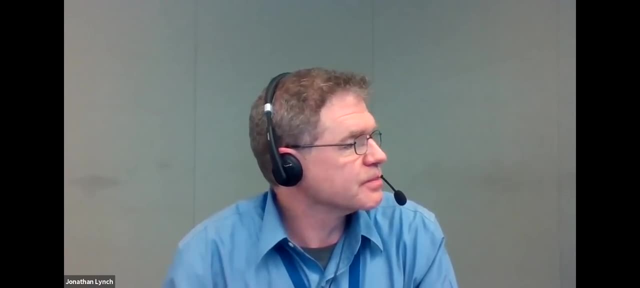 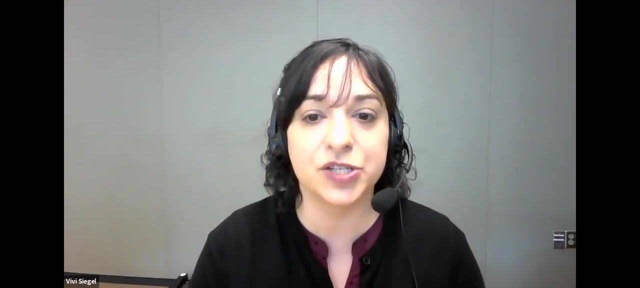 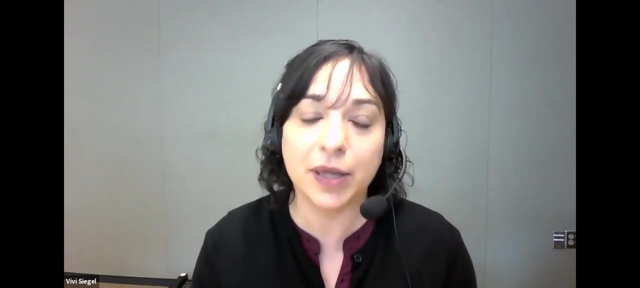 Vivi your thoughts. Thank you, John. I'm so happy to have you And I'm glad that you brought that up, because I do think that emergency management, PIOs and public health need to speak with each other on a local basis. 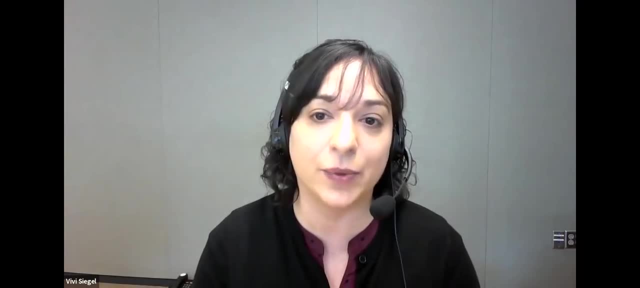 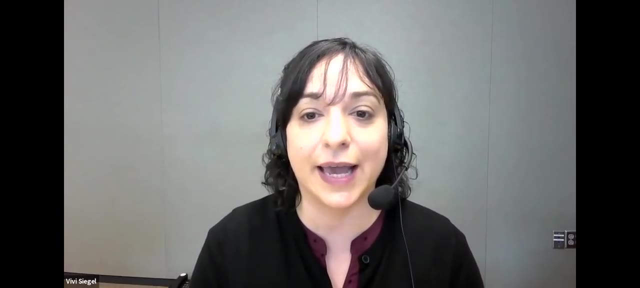 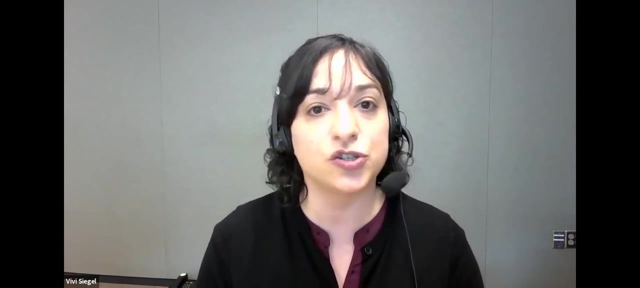 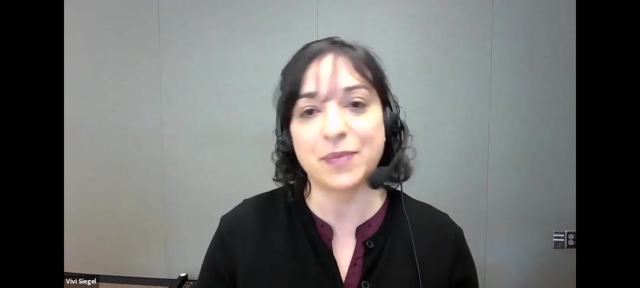 on a federal basis. We need to be close partners and we need to be talking with each other, often about how we can work together in a nuclear power plant accident, And I know that this is something that you guys train for and you have. Sorry, I'm having a. 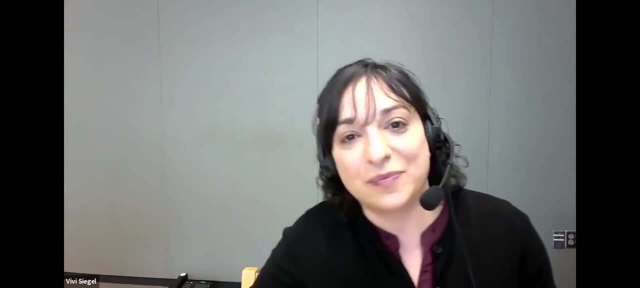 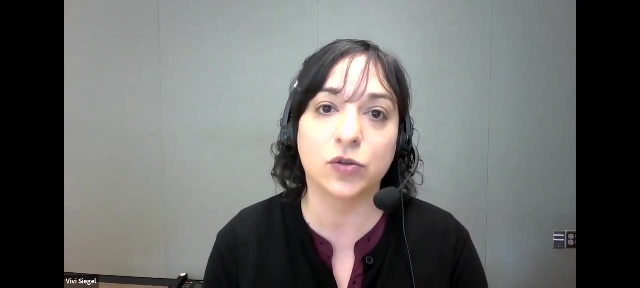 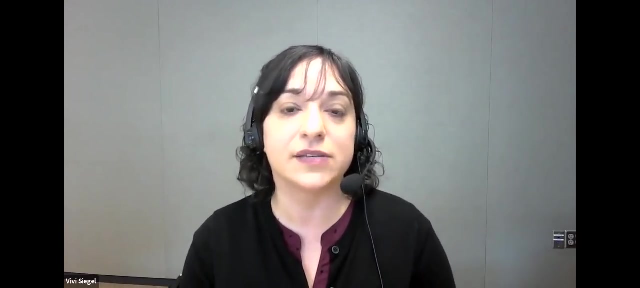 slow tongue right now, But that you have practice and I know that's certainly something that I would encourage folks who are having local exercises to make sure that public health is included in the exercises and involved and that there are lines of communication that are open. 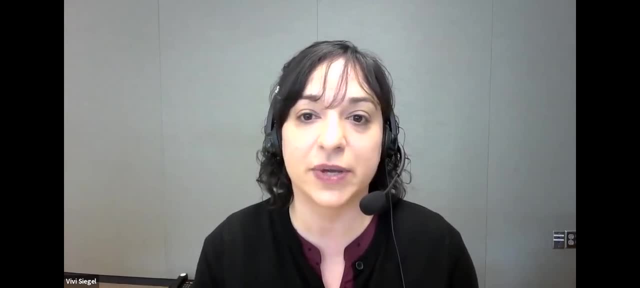 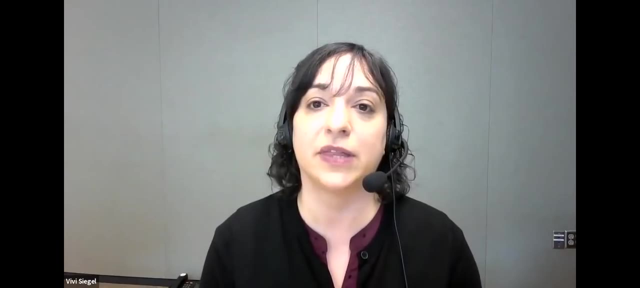 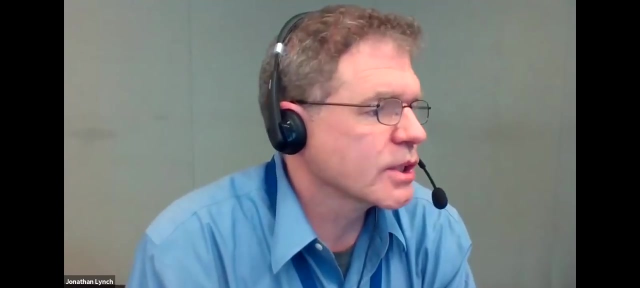 I was really happy to be at the National Emergency Management Association's PIO meeting in Atlanta last year to talk about this topic, and it's certainly something that we want to continue engaging with you guys about, So thank you. Okay, our next question comes from Vader, who asks: 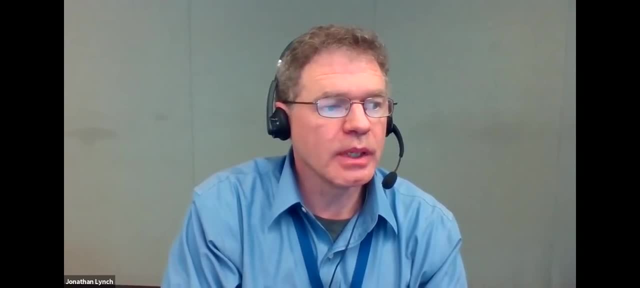 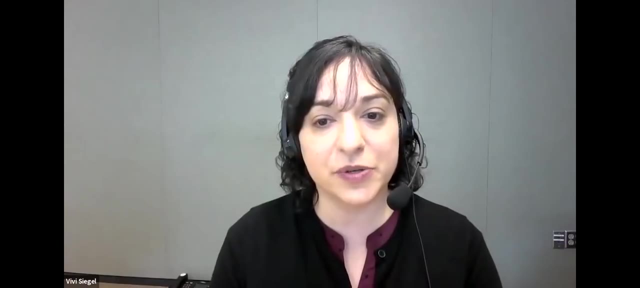 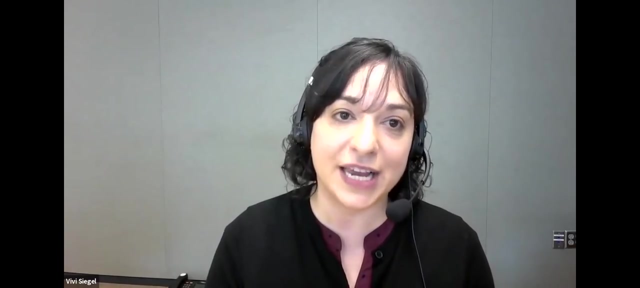 what is the level of radiation that can harm a human? Does the microwave have a negative effect on food? So that gets into some of those physics questions and again I'm not a health physicist but I can say that the amount of radiation from our microwave- remember we were talking about 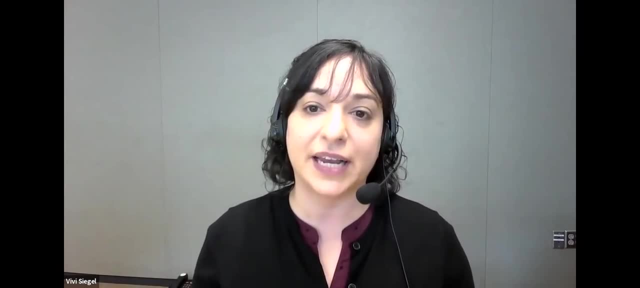 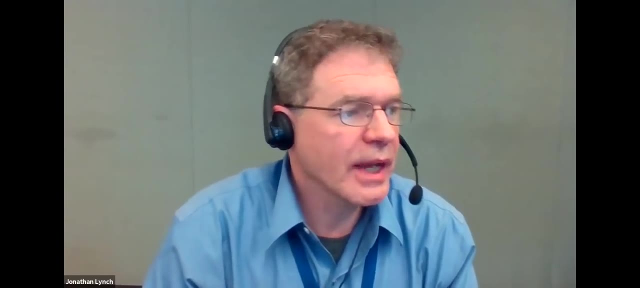 non-ionizing versus ionizing radiation. that's the type of radiation that can heat things out but that's not going to cause damage to our DNA And you can look at our. I would recommend checking out the radiation thermometer and it will go over what level. 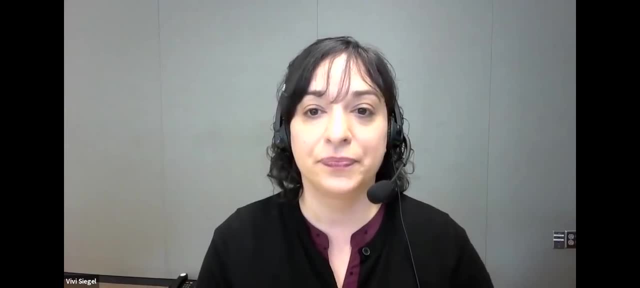 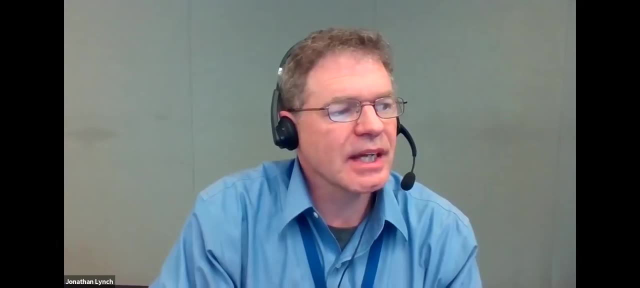 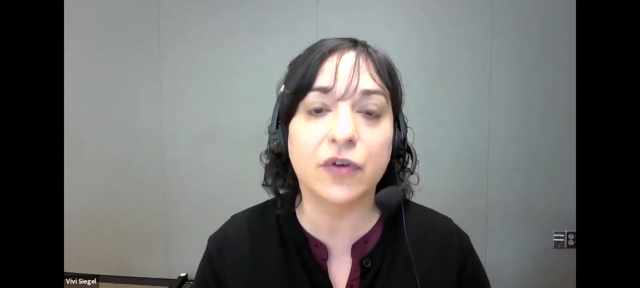 can cause health harm, Vivi. the next question comes from Robert Fisher, and this is a great question: Does CDC have guidance on decontaminating pets? Yes, so you can look at our infographics, and the decontamination infographic has information on decontaminating pets. 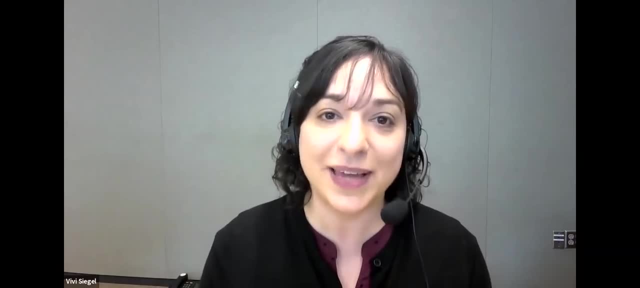 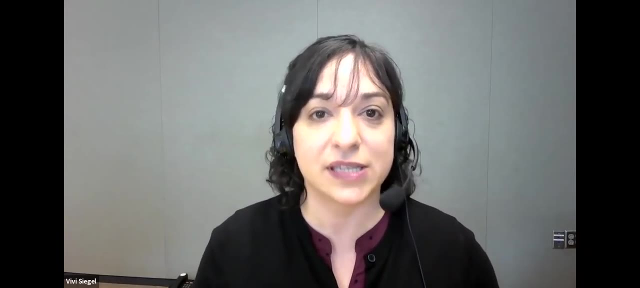 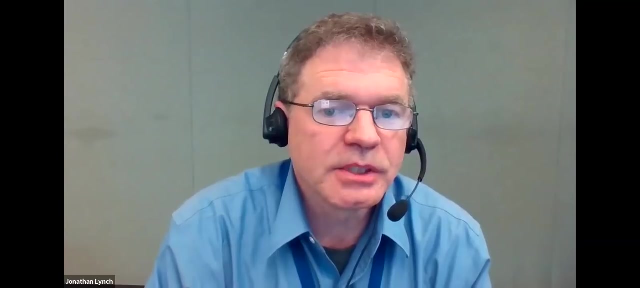 as well. It's very similar to what we do for people. It can be complicated because, you know, a dog has a lot of hair, and so there is information on the infographic about that, And our apologies to the audience. I know that there's been some. 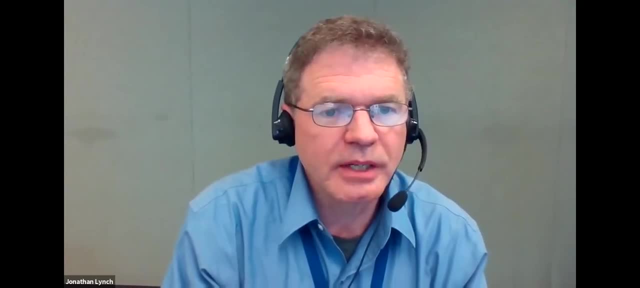 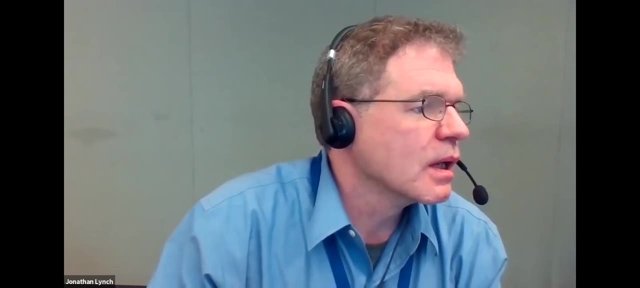 cutting in and out. It appears to be an internet connection problem kind of beyond something we can control locally. so our apologies for that. Adewale, I'm just going to go with Adewale for fear of pronouncing his last name incorrectly asked. 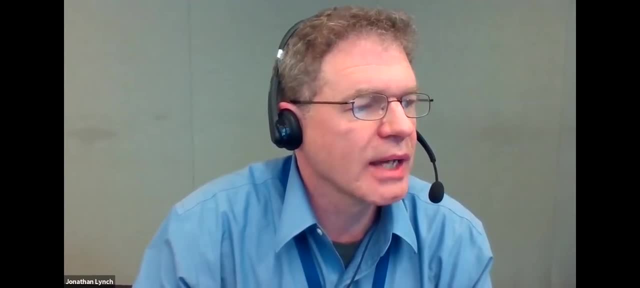 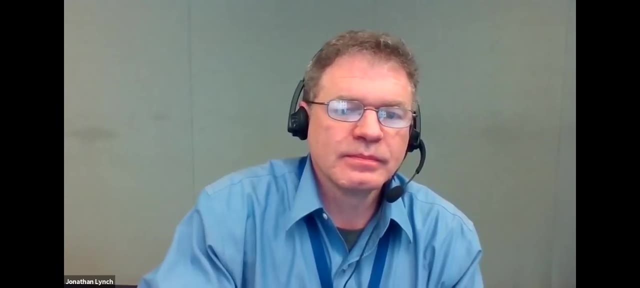 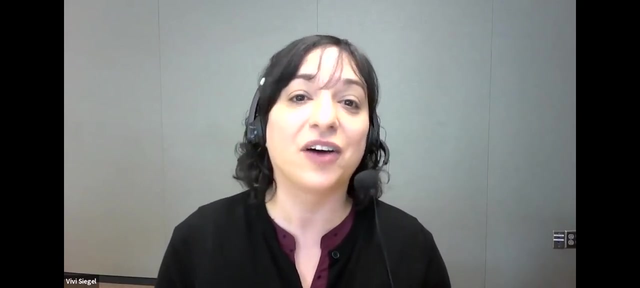 how about those exposed as a result of occupational hazard and continued exposure? What can be done to stem that? So that's a really interesting question and I don't know, unless we're talking about it might need a further conversation where we could talk more about the type of 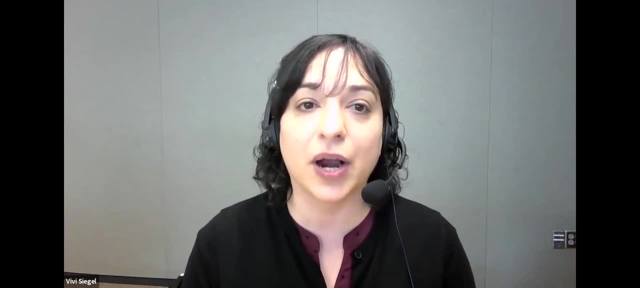 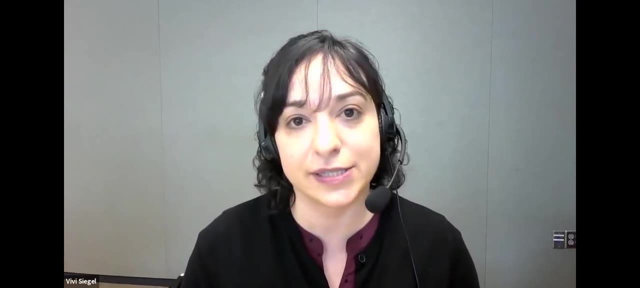 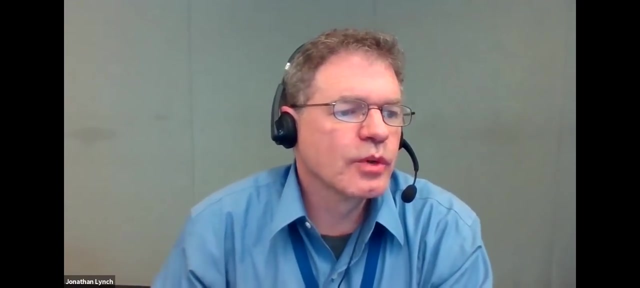 exposure, the length of exposure- But I know our partners at NIOSH, which is the CDC's center for occupational health, is definitely something that they are looking at and working on, Vivi. the next question comes from Harn DT, who asks: 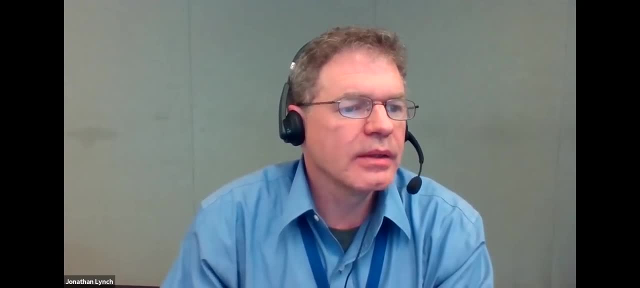 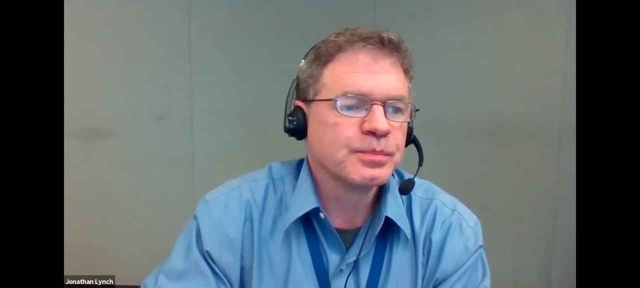 how is the CDC actively working with the state level public health departments for those states that have nuclear power plants? How are they involved with state EOC and state public health during nuclear power plant events? So, like with any type of emergency response, the federal 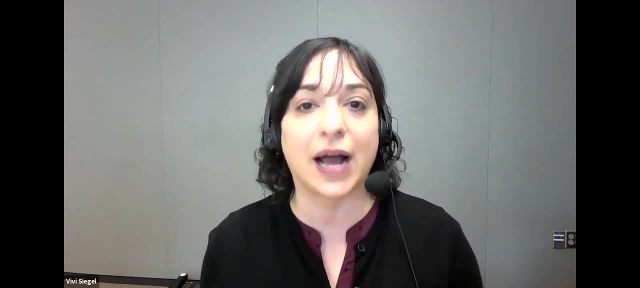 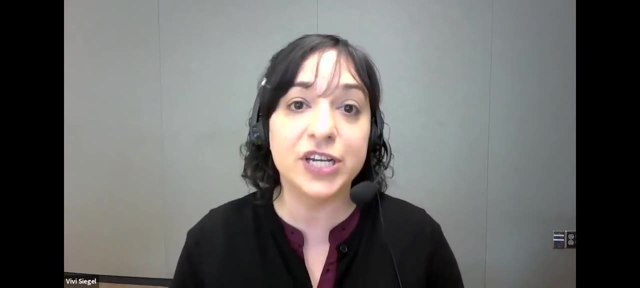 government would become involved if the state asked for support or asked for help. So if there were a case where there were a nuclear power plant incident in a state and the state reached out to the federal government for help or, in this case, if the state health department reached out to CDC. 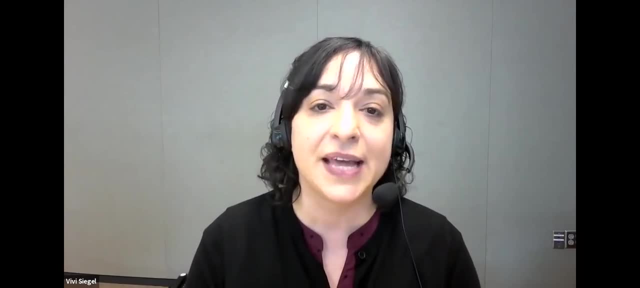 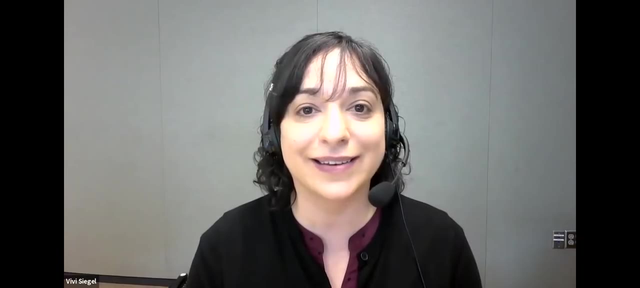 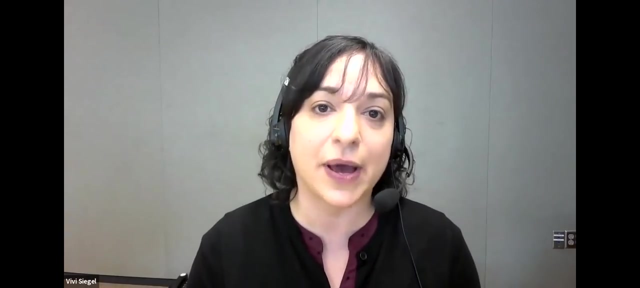 for support. we would be able to provide assistance As far as how we're helping as we go. over the last year we were happy to be able to sponsor a work group for state public health departments that had questions about communicating about radiation and nuclear issues. 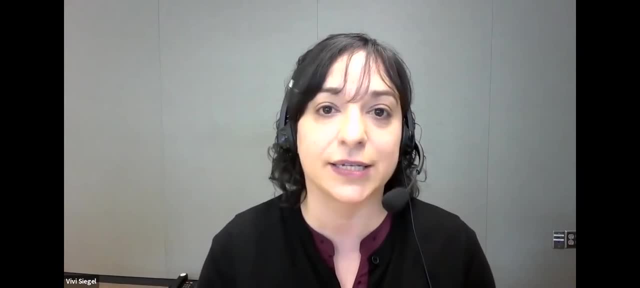 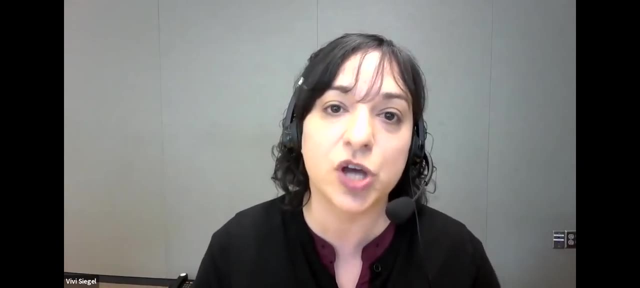 And so we had a monthly phone call and conversation, and power plants were one of the things, one of the topics that came up in our conversations and it's certainly something that we're open to talking about more and thinking about other ways that we might be able. 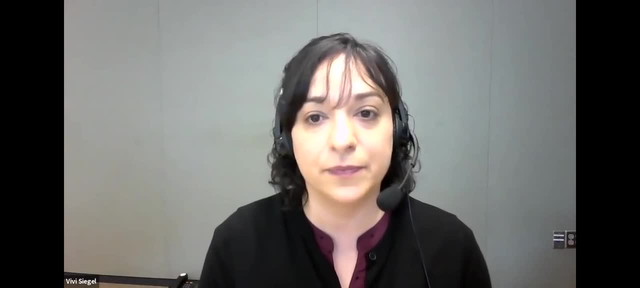 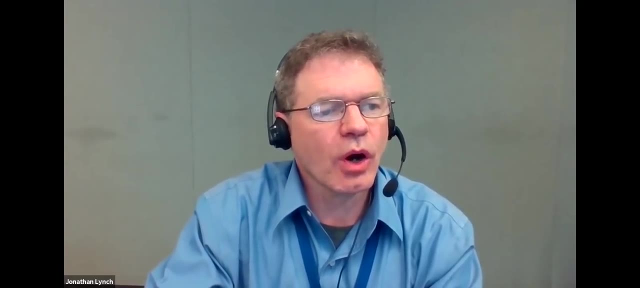 to provide support if needed and if that's something that's requested by a state. I'm looking forward to that. Our next question comes from David Cal, who asks: seafood caught off the California coast in recent years has been found to contain radioactive contamination from the Japan-Fukushima nuclear. 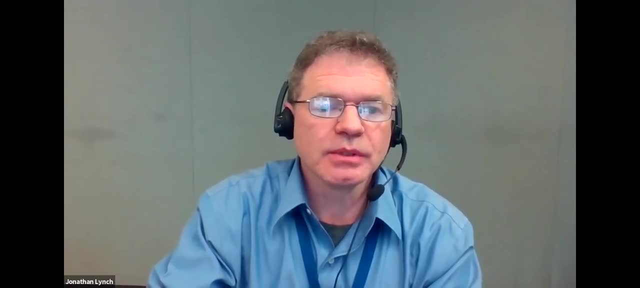 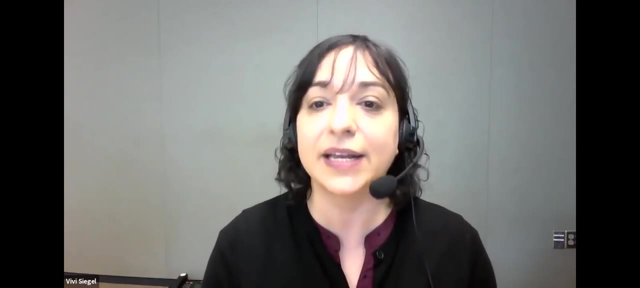 power plant disaster. Is this seafood safe for human consumption? So this is not something that I've been involved in working in, and so I don't know that I'm the right person to necessarily give that answer on what's safe regarding seafood to eat and not to eat. 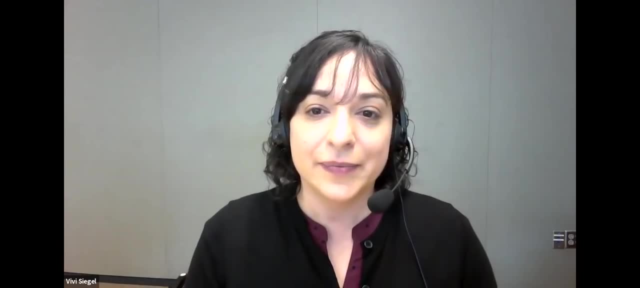 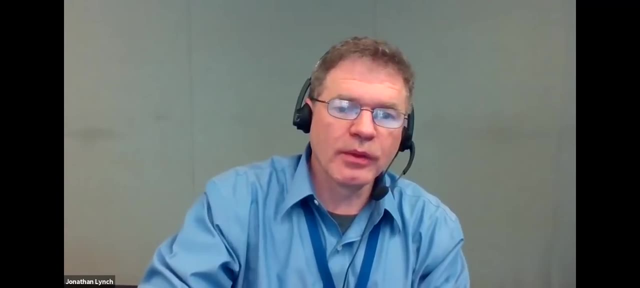 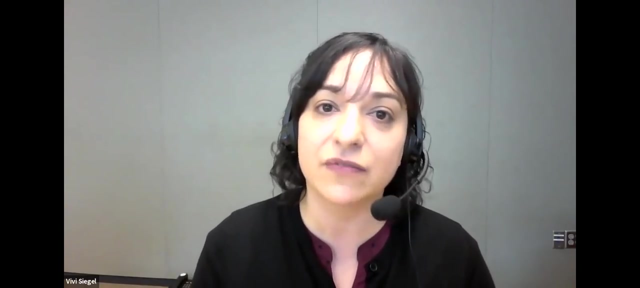 However, it's not a health risk to my knowledge. If they wanted to learn more about those specific topics, I can definitely look into where you might be able to find out more about that and get back to you, but that's not something that I have. 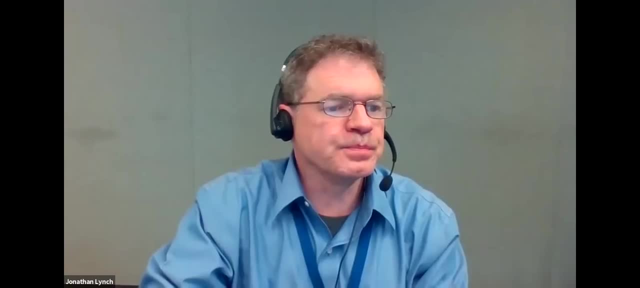 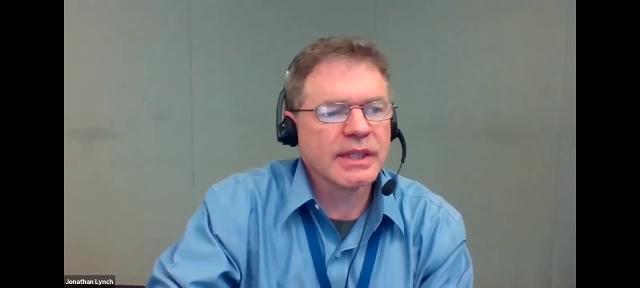 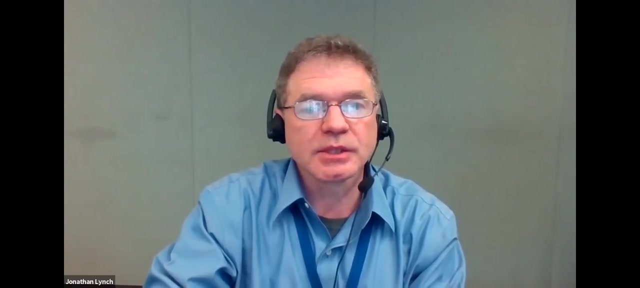 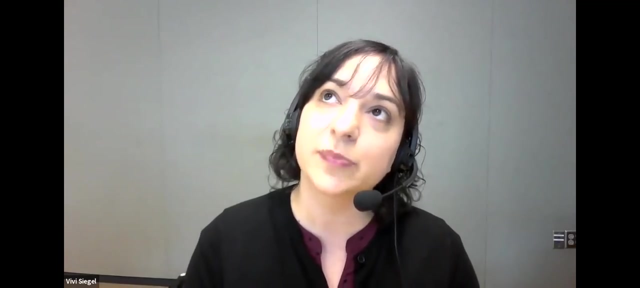 any more information on. So our next comment comes from Craig Heffron, who says: is there a standard infographic slash information sheet that first responders can quickly and easily provide to survivors to enhance the six principles? Is there a standard infographic or information sheet that responders could use? 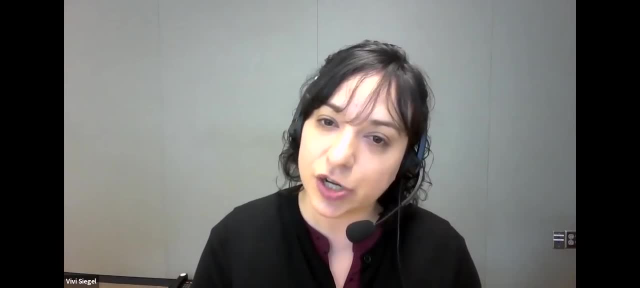 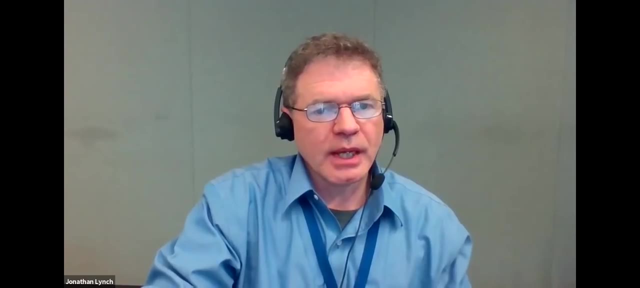 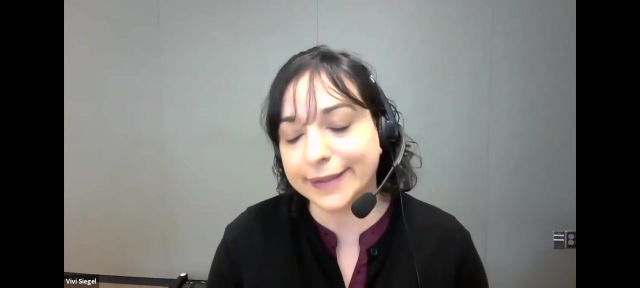 to emphasize the six principles. The way I would interpret that is, following those six principles, what would be the infographic that would most address the concerns that the six principles call upon us to address? Absolutely. You can go to the link and see the infographics. 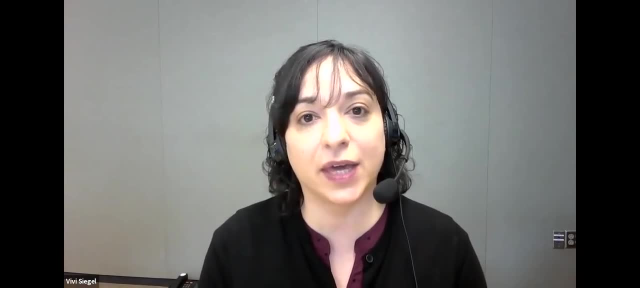 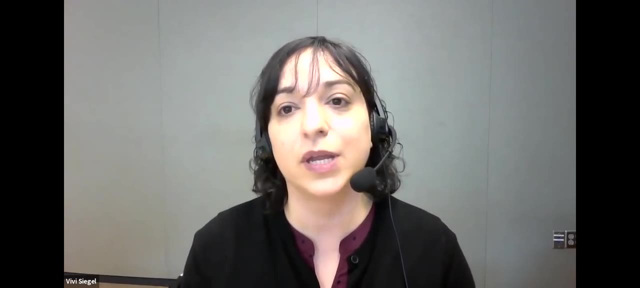 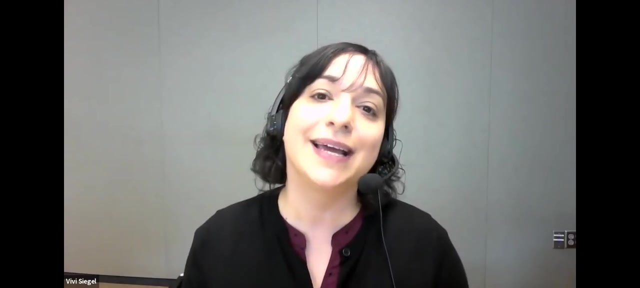 that we do have available. I think the biggest principle in CERC that we'd want to get out there right away is: what are the immediate actions that people need to take? Like I said, this is something that's going to be difficult to sometimes get to someone. 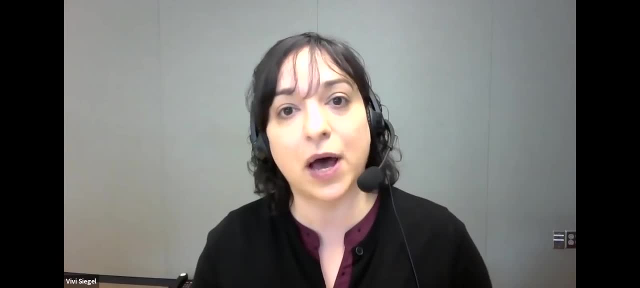 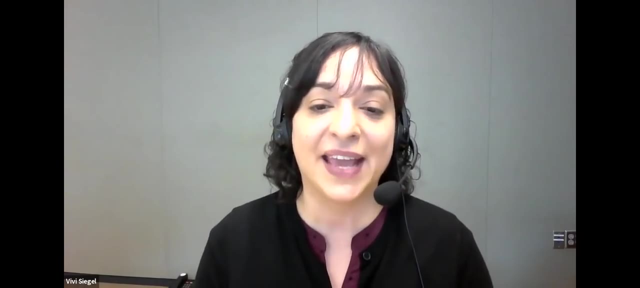 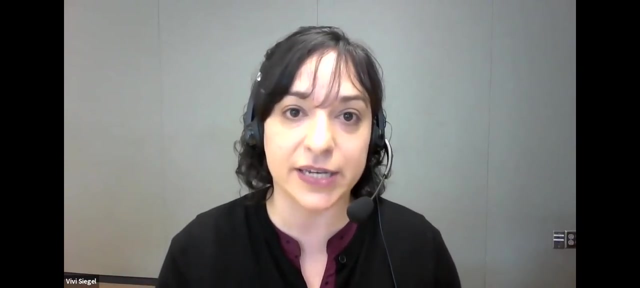 who's experienced an accident. Some of this is about education beforehand. Do they need to know how to find information? Do they know that this type of information exists? Some of it is being able to get it to them through all communications possible in an event. is getting 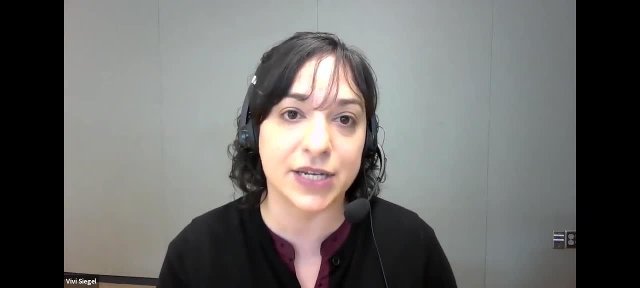 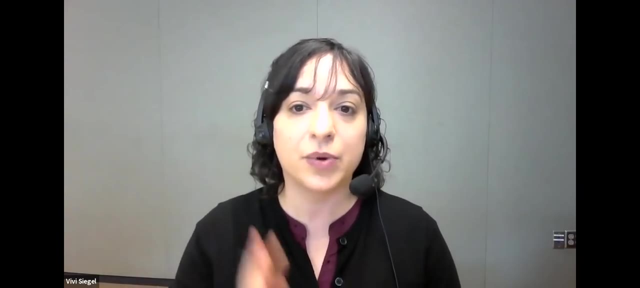 them that first protective action: Get inside, stay inside, stay tuned. Everything else after that is secondary. That's the most important message to get out. It's got that protective action and we want to get it to them first. Obviously, we know it's an accurate. 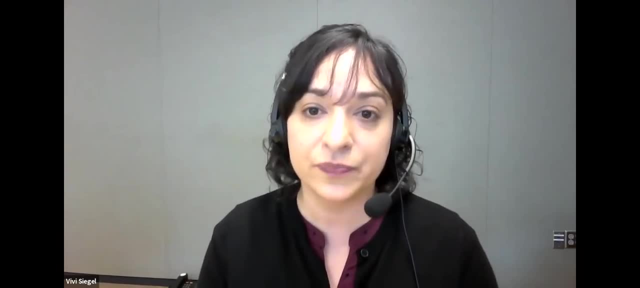 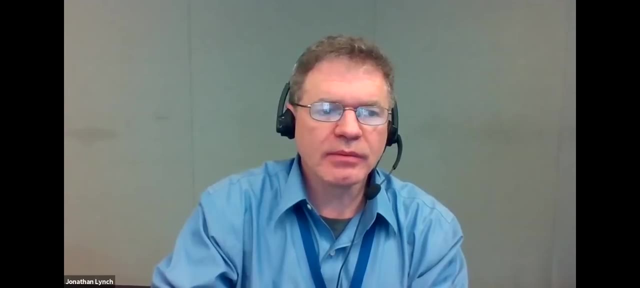 message and we hope that it's credible and it's coming from a credible source. Thank you, Vivi. Shannon Seneca asked: is it more important to be at the lowest level in a building or away from windows? because of the fact that most 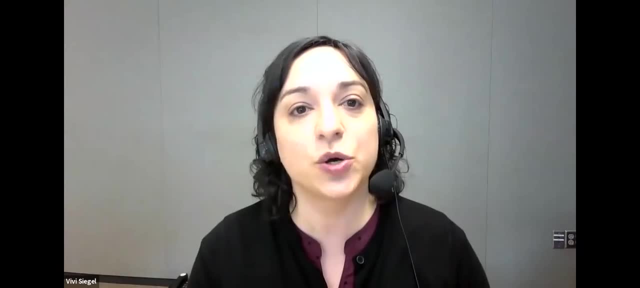 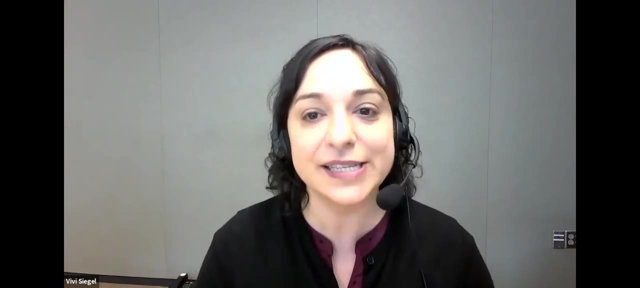 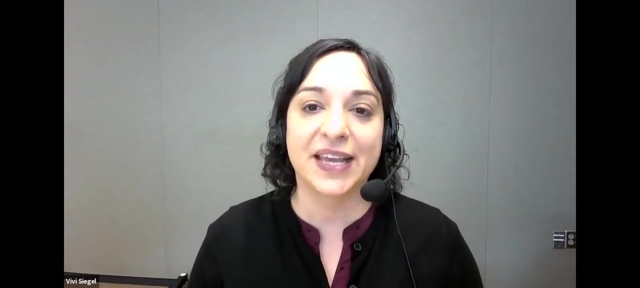 basements have windows? That's a really good question. I would actually turn to some of the infographics that you can find from some of our partners that really show. EPA has a really good one that shows the protection factors of different parts of a building and 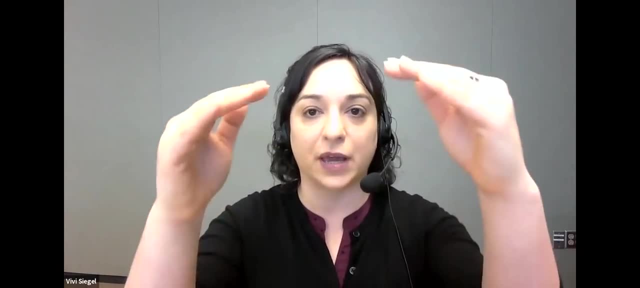 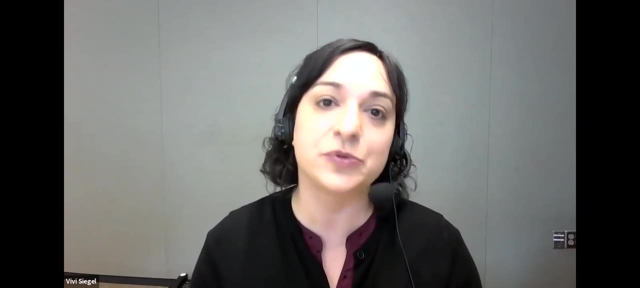 certainly there's some risk by being next to a window. there's some risk by being higher or lower, and I can't tell you off the top of my head what's the worst risk, but I know there are people who study this and can tell you what angles. 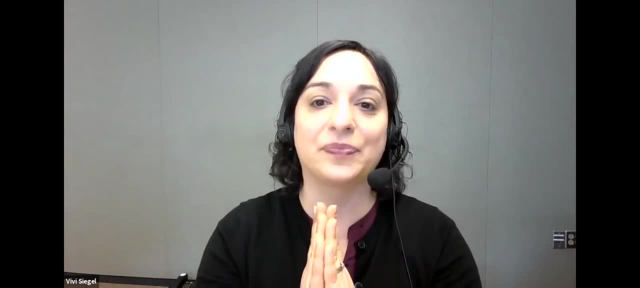 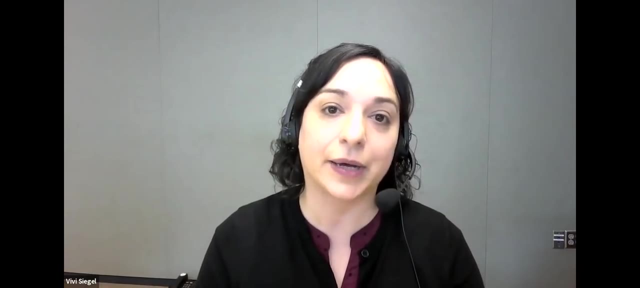 you need to be away from the window? The basic answer is: away from the windows and underground, if you can. So if you're in the basement, go to the middle of your basement, the farthest you can get away from the windows in the basement. 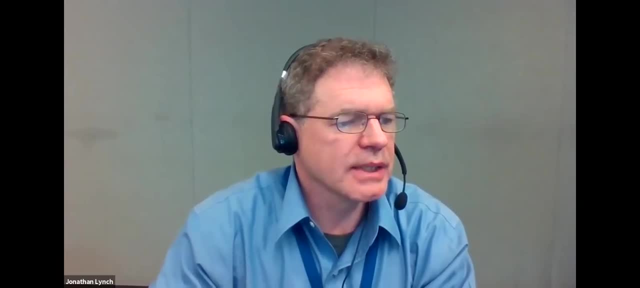 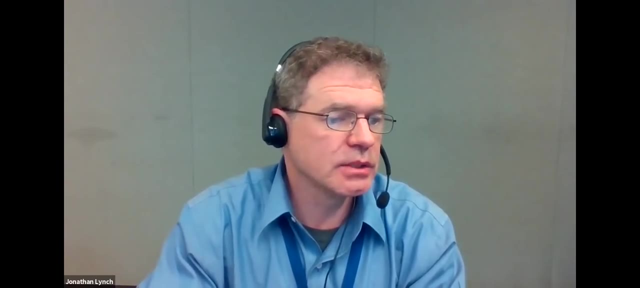 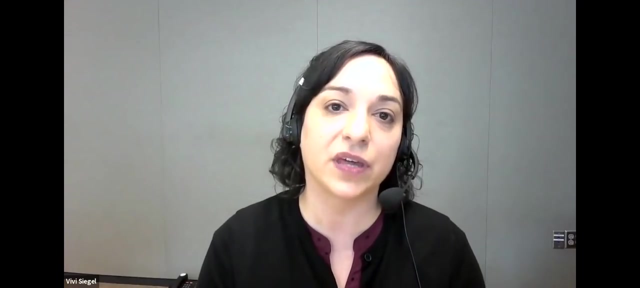 We got a question from Katerina G who asked: is there any difference in the communicated actions regarding shelter in place versus evacuation dependence on the distance to the radiating source? Yeah, so that's a really good question and that's going to be something. 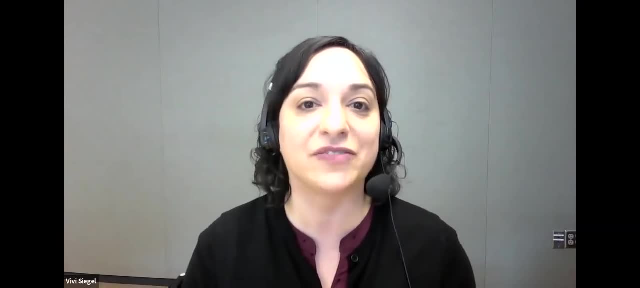 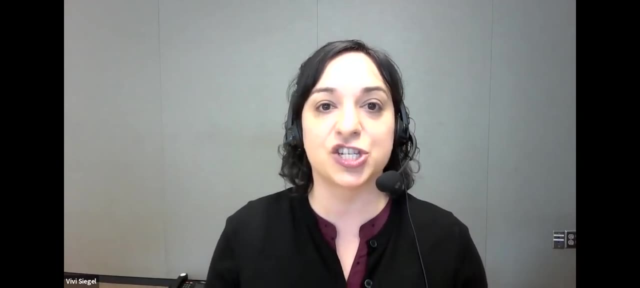 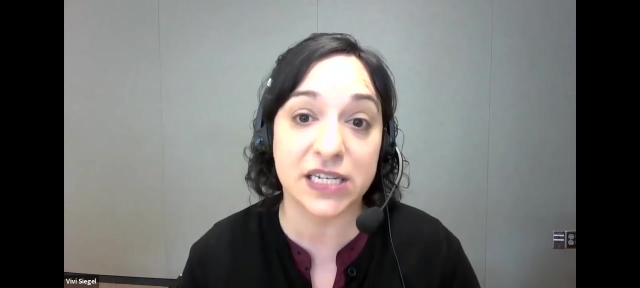 that health officials and emergency officials are going to have to determine in an event like this is: are there places where people should be evacuating versus sheltering in place? The quickest answer is that sheltering in place is probably going to be the protective action that's first given and then 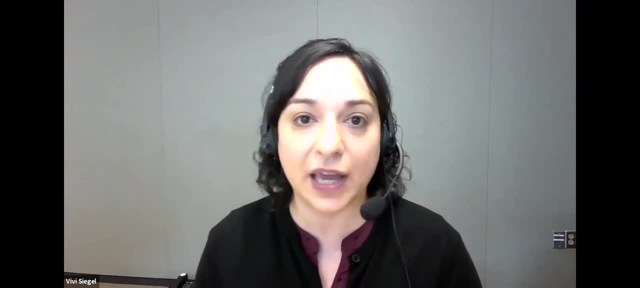 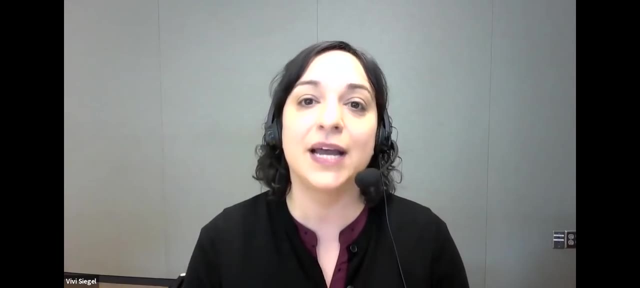 decisions will be made about if it's safe for anyone to evacuate and where they might evacuate, to who should evacuate. but assessing all of that is going to take some time, and the safest place for people to be while that's being figured out is going to be. 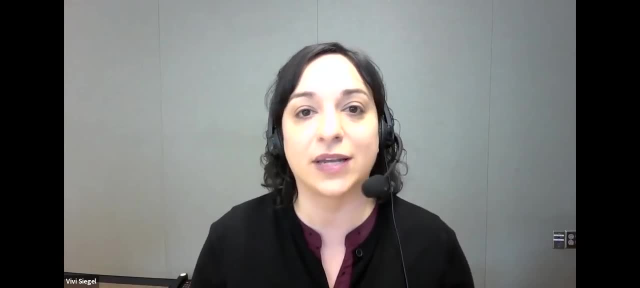 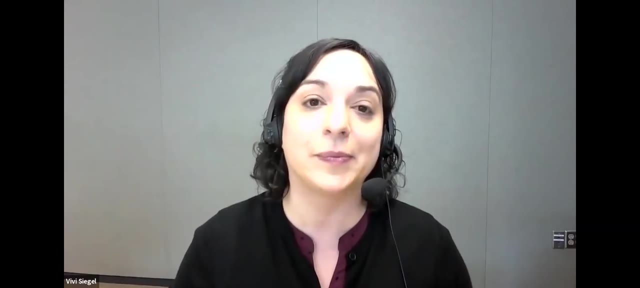 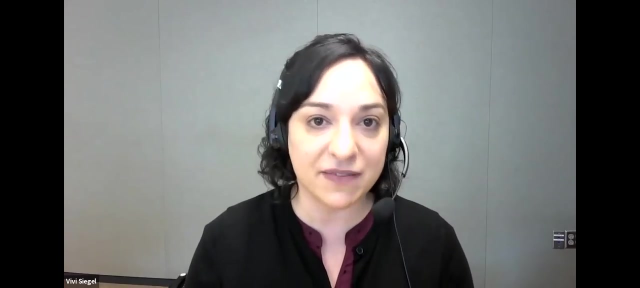 inside sheltering in place. We also don't know, based on atmospheric conditions, wind models, where the contamination might go, and so, whereas someone might think they're in the clear to evacuate and step outside, they might find after they get outside that it's not safe after all. 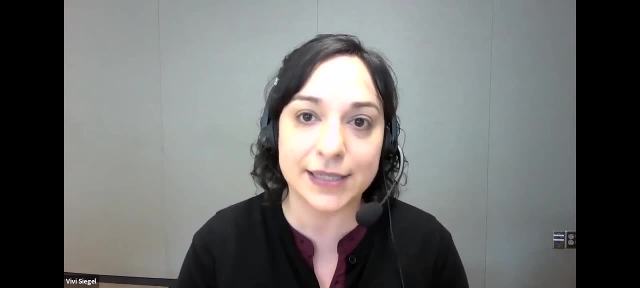 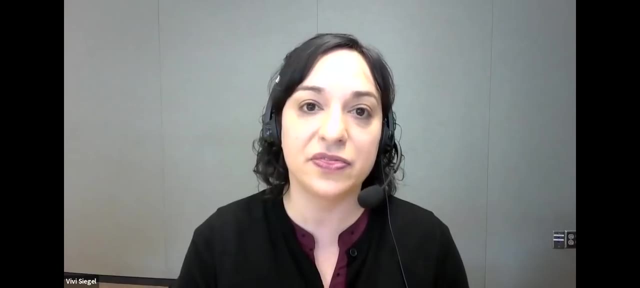 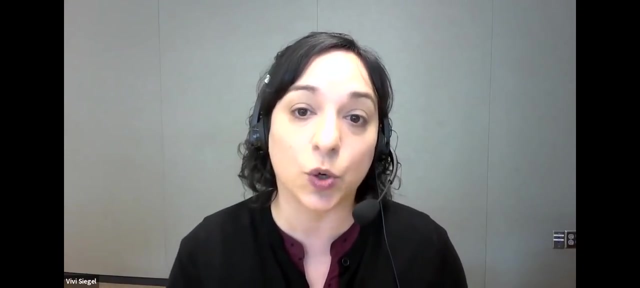 so we do recommend that the first message is: get inside, stay inside and then, when we have more information, then think about potential evacuation. And that again, is going to be like all evacuations and emergency decisions: that will likely be a decision that's made at the local level. 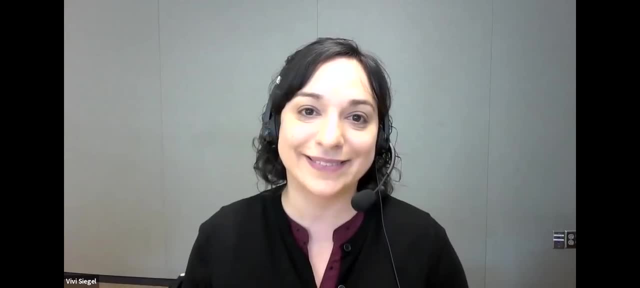 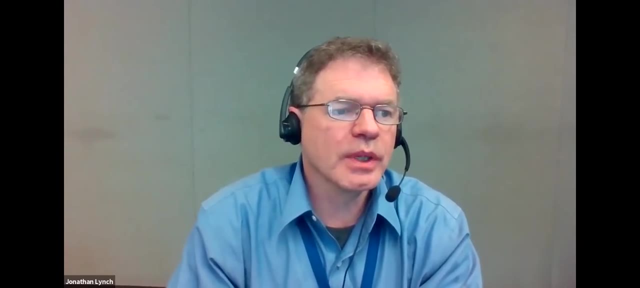 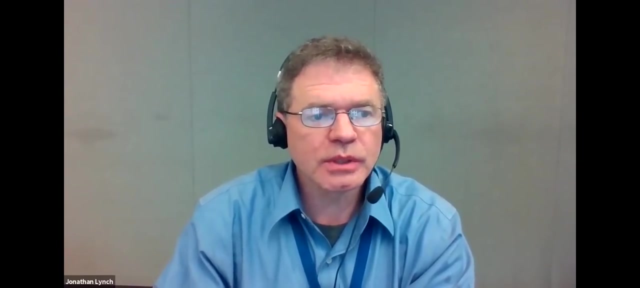 as to where, how those evacuations will work and what they might look like. Okay, Two more questions. The first one that we're going to address is from Alejandra Maldonado, who asks: are there guidelines or resources to coordinate communication with the local? 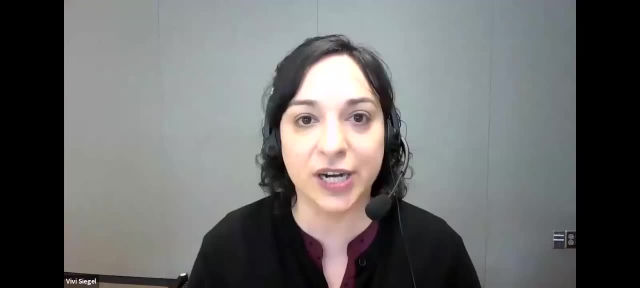 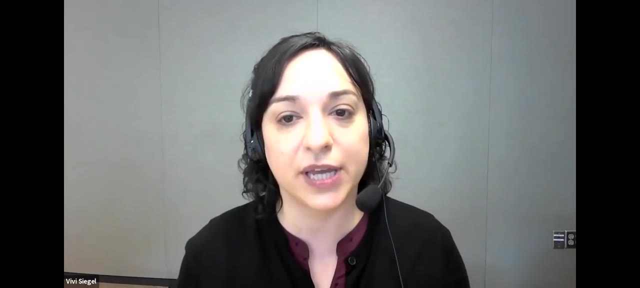 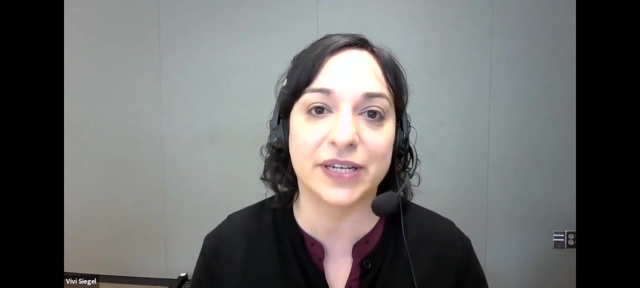 media to prevent misinformation. Sure, That's a really good question and that is something that we address in the crisis and emergency risk communication. training is how to work with the media. One thing that I find to be useful as a former member of the media is I really believe in creating. 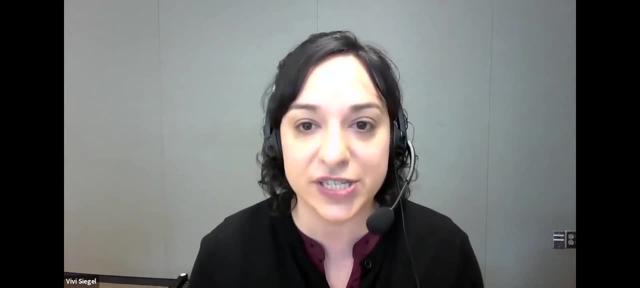 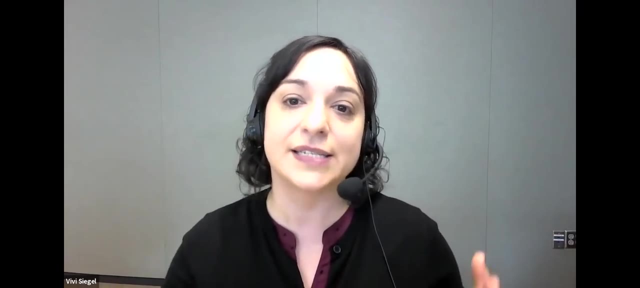 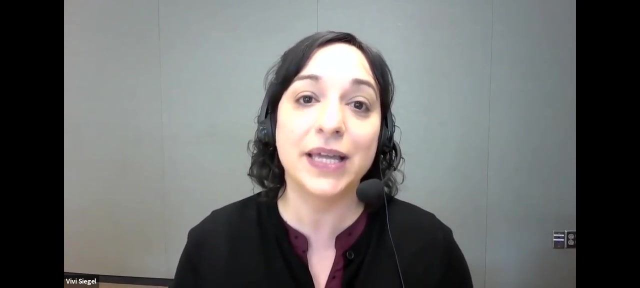 strong relationships with local reporters who are interested in the topic, Doing some of this education before something like this happens, so that you're both positioning yourself as an expert source, so they know who to come to in case something like this happens, and it'll save some time in an emergency. 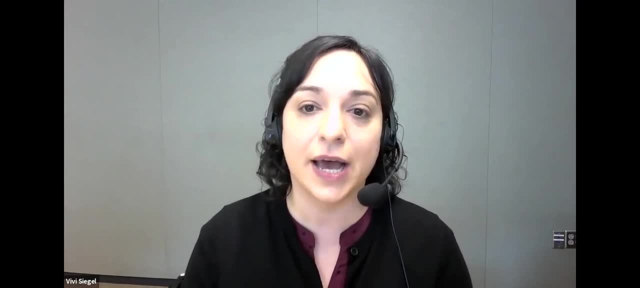 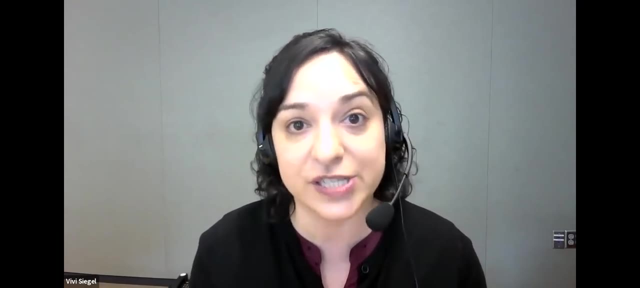 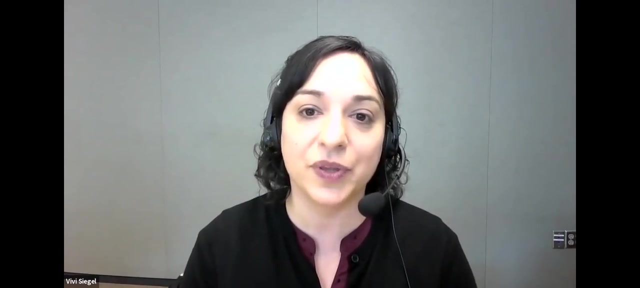 because they'll already know our emergency recommendations. I'm a strong believer in working to build media relationships and build trust in non-emergency situations. As a former mentor of mine always said, you don't want to be exchanging business cards while the emergency is happening. You want to already know each other. 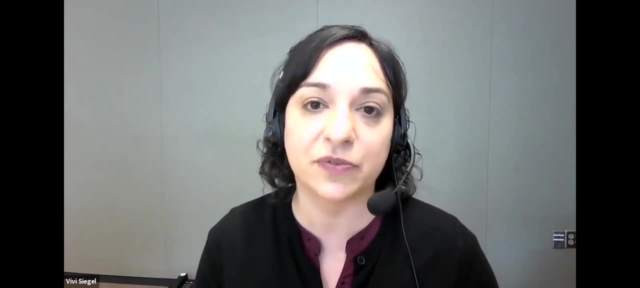 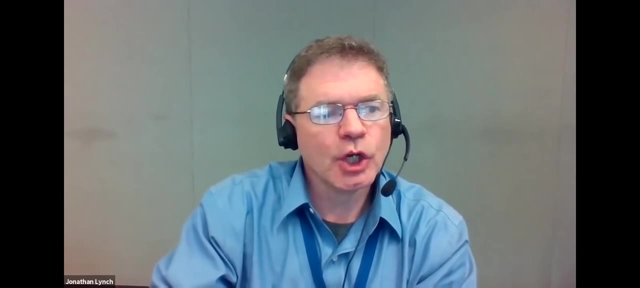 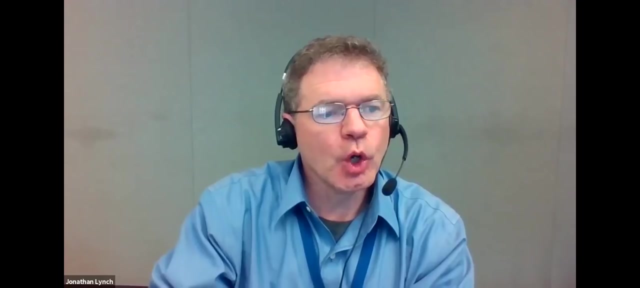 and be working on that building trust beforehand. Our last question comes from Bonnie. I work in pediatric triage. During the Fukushima incident and North Korea threats, we had parents calling panicking about what to do. Who would we refer them to in such a situation? for? 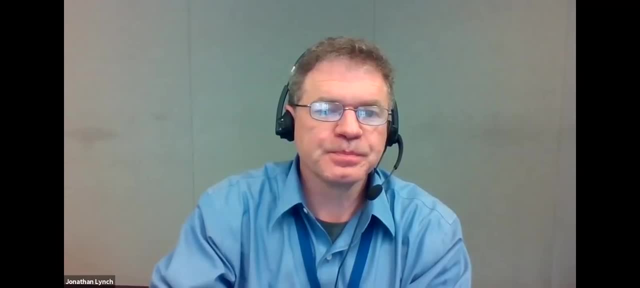 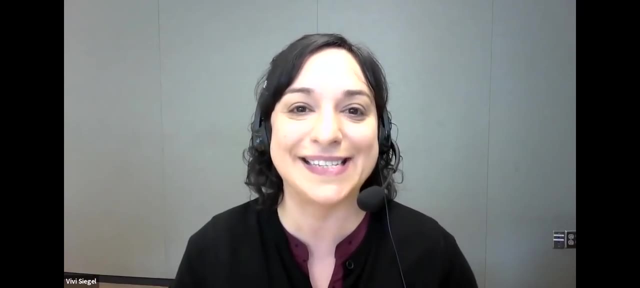 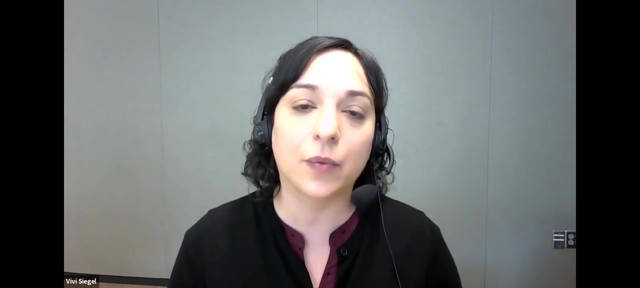 appropriate information. Thank you, That's a good question. I don't know right offhand. I know that during the Fukushima response, CDC did have- and we often have during different emergency responses- we'll have a physician hotline where physicians can call to get information. 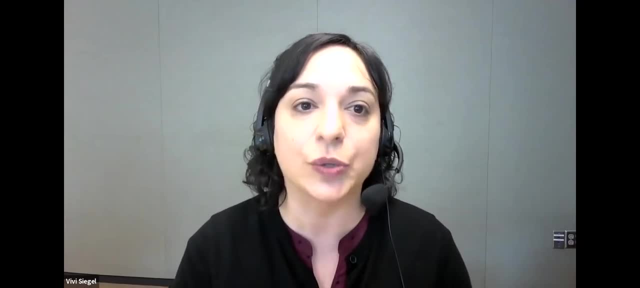 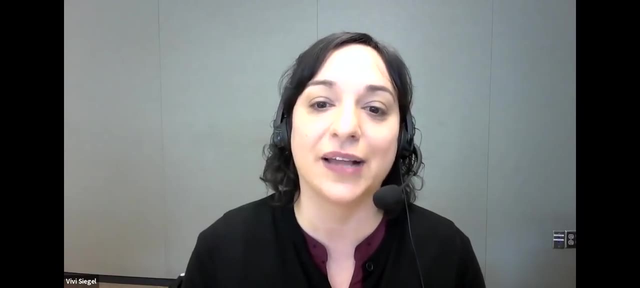 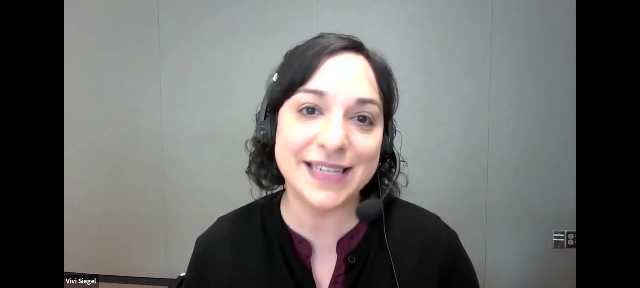 and find out where referrals can be made if they need to. My hope is that you'll have you would be able to refer them to CDC's website or local or state public health department website. that would have clear, accurate, easy to understand information that would help. 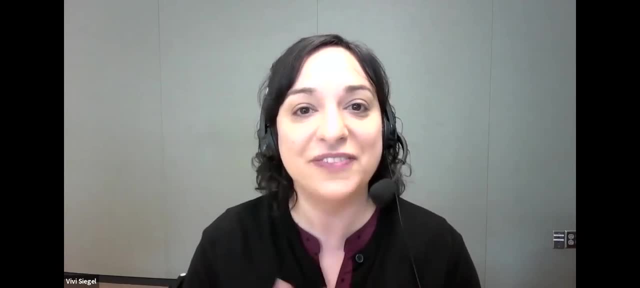 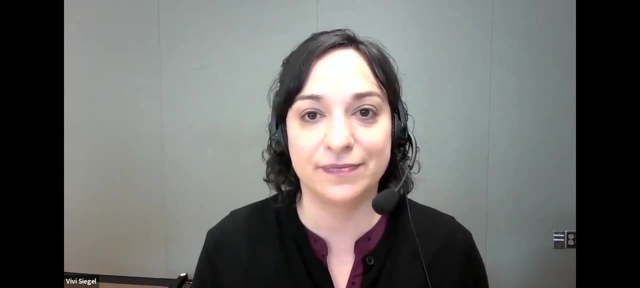 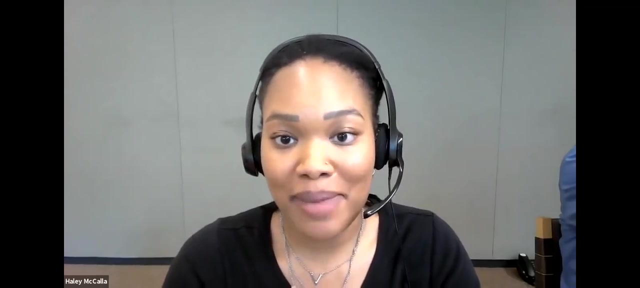 answer some of those questions. I know that myself and the folks on this EPIC team would be working to help make sure that information was available to you. Thank you, We'll now conclude our Q&A session. I want to thank everyone for all your participation. 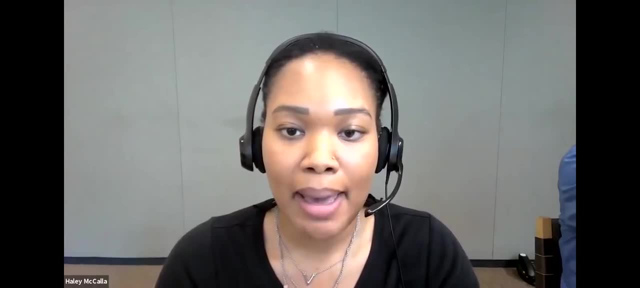 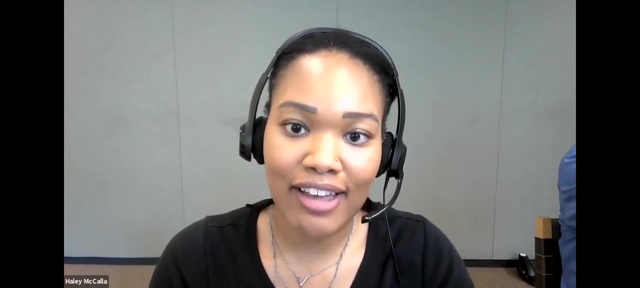 We had a lot of comments and questions that we weren't able to get to today, but if you would still like an answer to your question, please email us at epic at cdc dot gov, and we're happy to wrap those questions to Vivi. 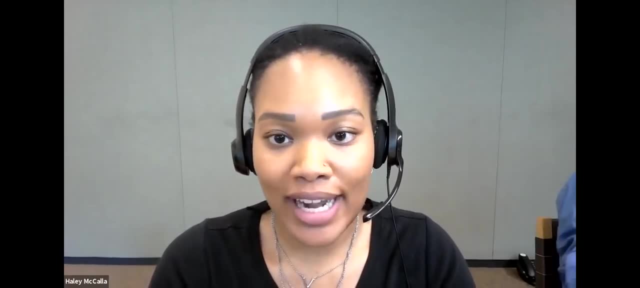 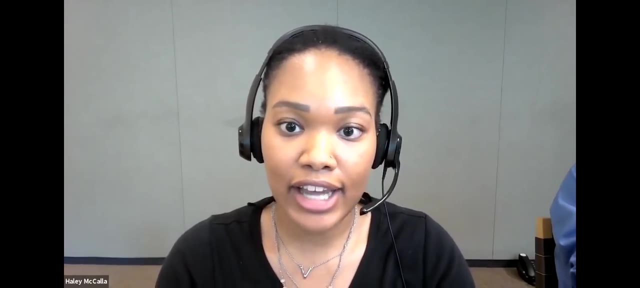 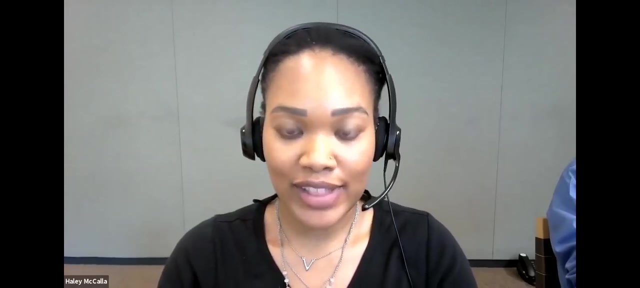 As a reminder, today's presentation has been recorded. The slides are available on the website at this moment. Once again, our website is emergency dot cdc dot gov. so those slides are available for your review. For continuing education. you can earn that for. 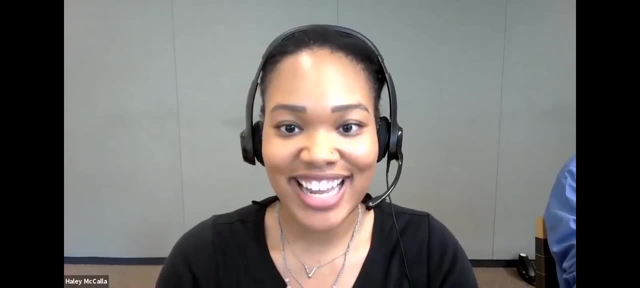 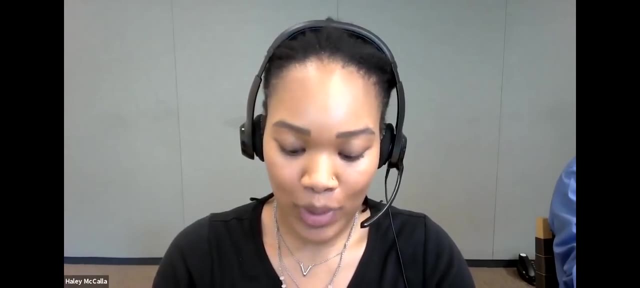 participating. so please follow the instructions found on emergency dot, cdc, dot, gov, slash, epic, and the course access code is EPIC 0227 with all letters capitalized. Thanks again, everyone. Have a good day. Thank you.